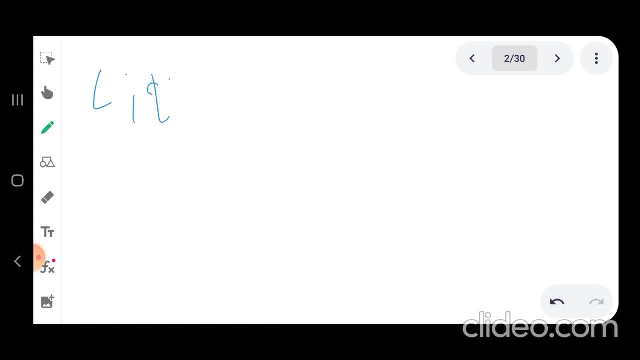 liquid. liquid, it's a vase. it's a vase. that's a type of fluids. no fluids. any fluid could be gas or vapor or liquid. okay, so our focus in this chapter is only on liquids. it's not like distillation, where you see liquid and vapor. no, for extraction, for this chapter I'm going to focus. 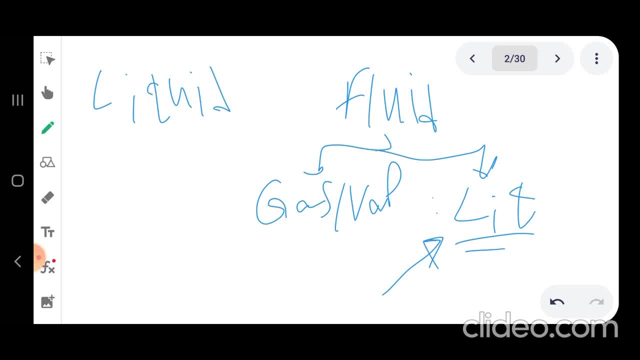 only on the type of extraction called liquid, liquid extraction. so it involves only liquid phase. okay, the question here: does liquid phase- is only one phase? always? the answer is no. you can have two different liquid phases. so what's the meaning of a vase? what's the meaning of? 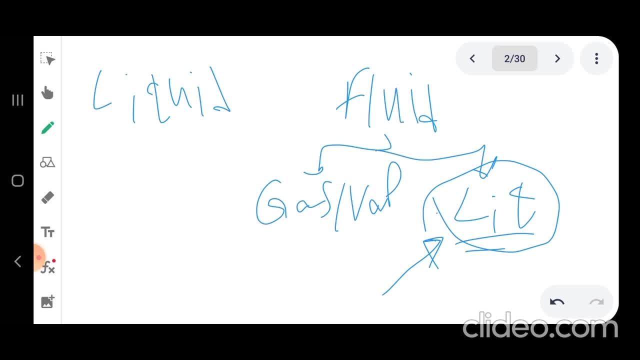 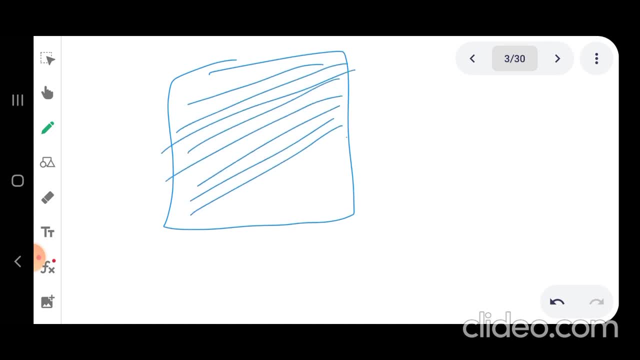 vase. so vase vase is just a homogeneous, homogeneous matter. homogeneous matter: what do we mean by homogeneous? homogeneous means? it consists of three things: constant temperature, constant pressure and constant composition, composition or concentration. to better illustrate the concept of what do we mean by a vase and how we can have two vases and both: 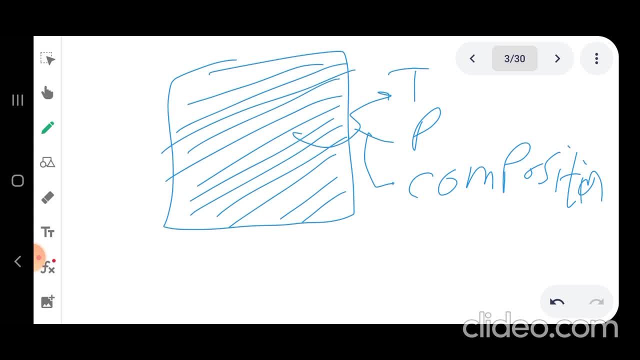 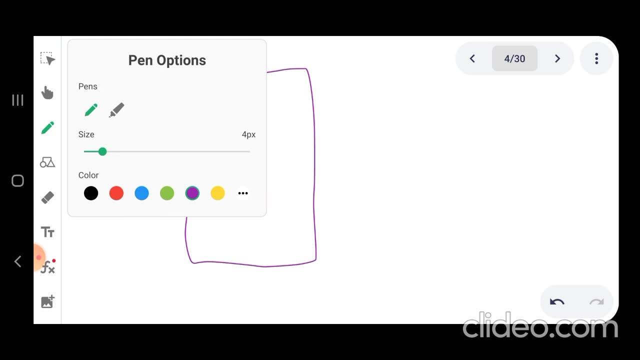 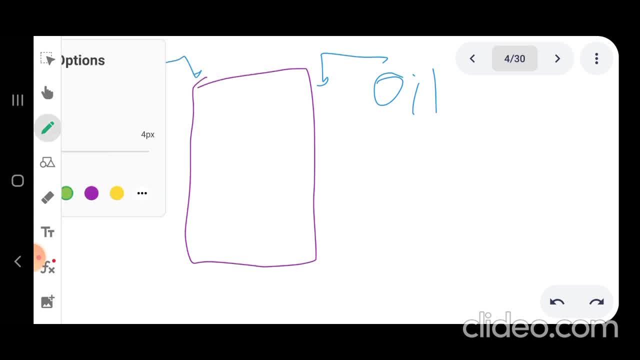 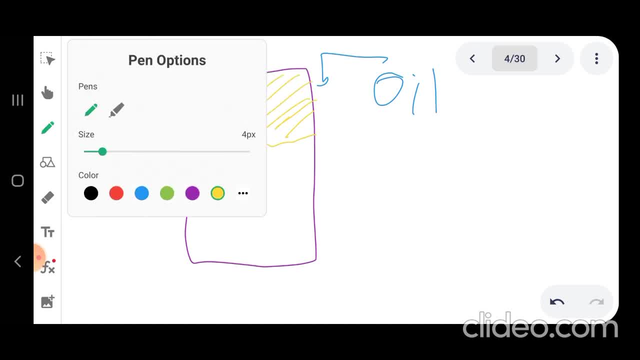 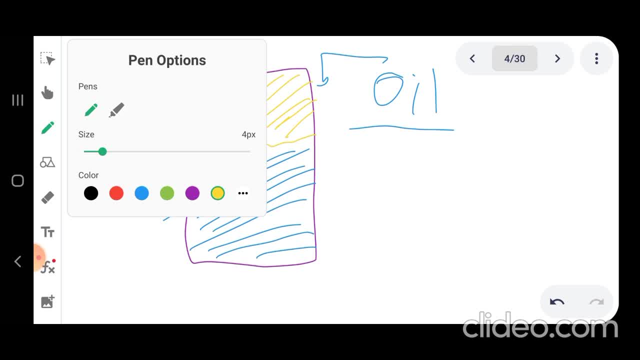 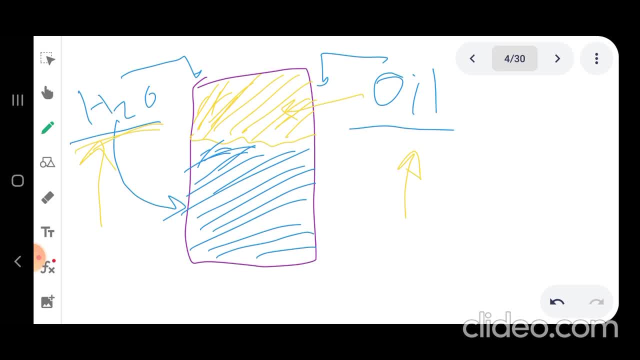 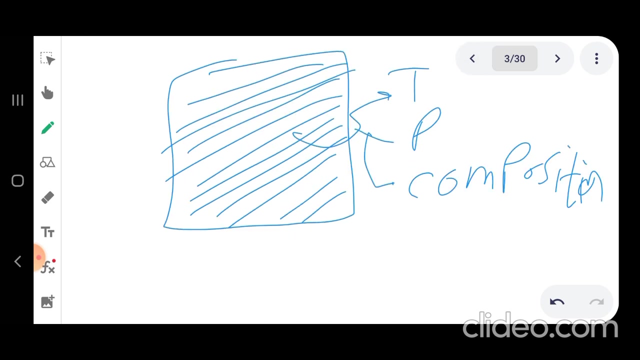 higher density. okay, so another question here to be asked is how many vases we have inside this system- oil and water system. how many vases? the answer here lets back to the definition of what a vase is. as we said, a vase is a matter that has constant temperature, pressure and composition throughout. okay, so if we 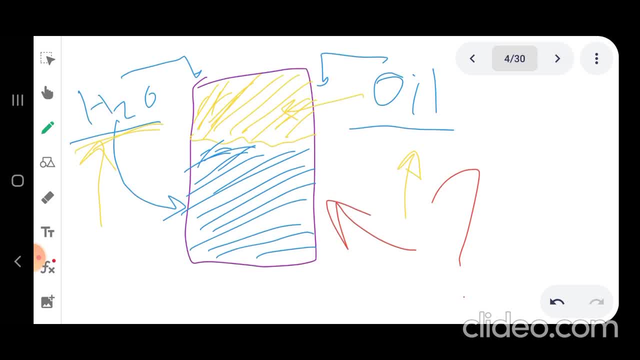 see if we look at this system. suppose, for example, that the temperature in all of the container let's say 25 degrees C ambient temperature and one atmosphere ambient pressure. let's support this in the temperature and the pressure. so so far, let's say: and now we have the same. 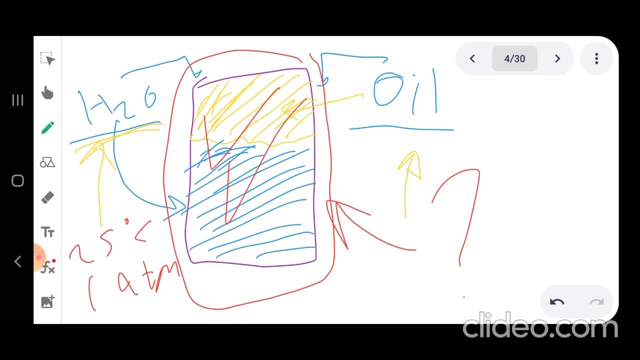 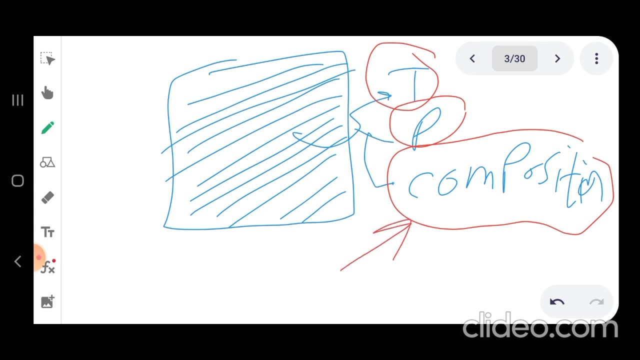 temperature and same pressure throughout the whole container. so so far we have only one base. we have only one base, which is liquid base. okay, but now let's see the third restriction here. the third restriction say that in order to have one base, you need to have the same composition everywhere, the same. 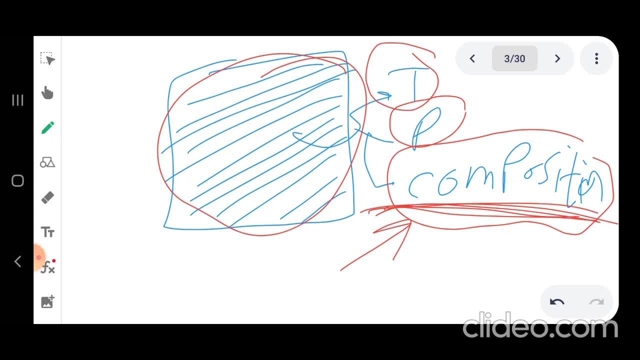 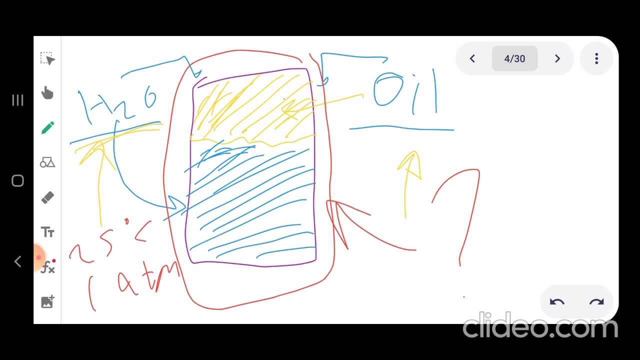 composition and the same chemical makeup. okay, but if we look at this container, we would find that the composition here at this point is different than the composition here at this point. why is that? because let's say this is point 1 and this is point 2. at point 1, everything is everything is oil, almost. 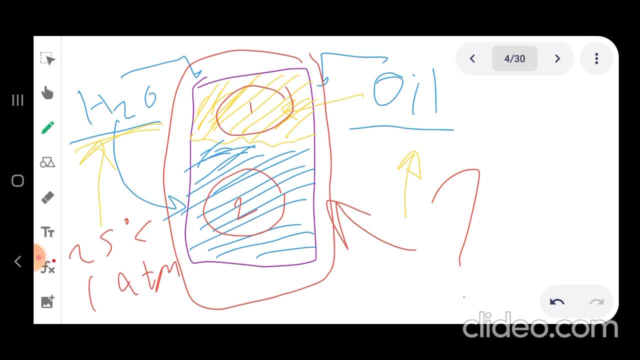 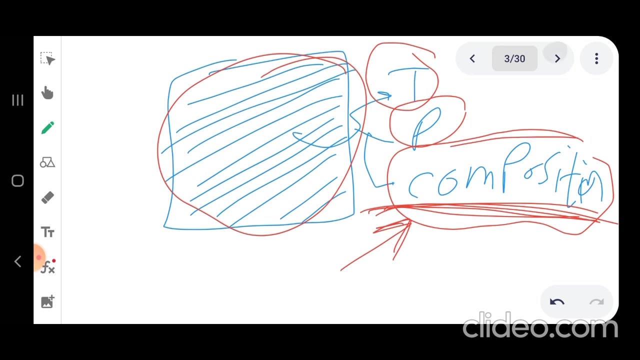 maybe you can have some three, three, three 's small amounts of water, but mainly at point 1 this is oil, but at point 2 this is mainly water. you can have some traces of oil, but mainly it is what it is: water. so you can see, you can see here that we violate the third restriction. I, here, we 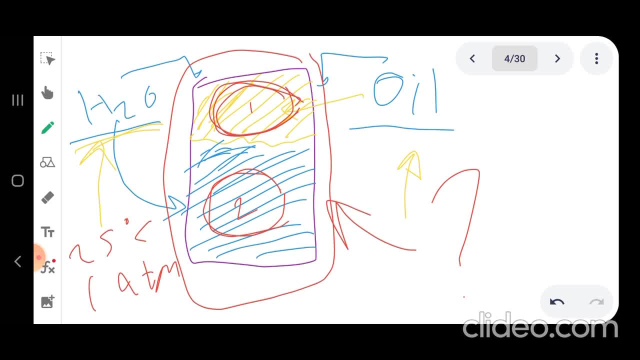 have a different composition, which is mainly oil, and there we have different composition, which is mainly water. so we can consider each of these as one base, each of these. in other words, in this system we have two bases: one base that contains mainly oil, another base that contains mainly H2O oil or water. okay, so you can see, here we still have. 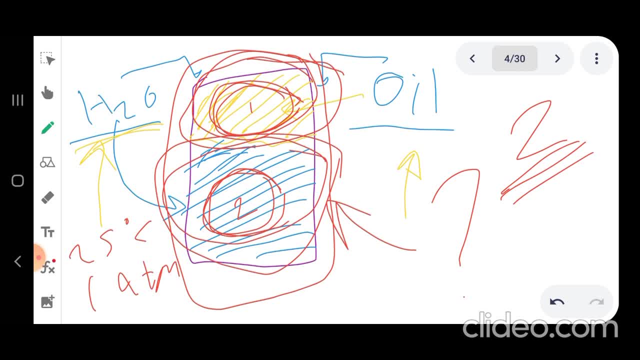 have liquid base. it's a liquid state. let's say to not confuse you. let's say it is liquid state. so we still have liquid state. oil is liquid and H2O is liquid. but we have two phases. why we have two phases? because we have a. 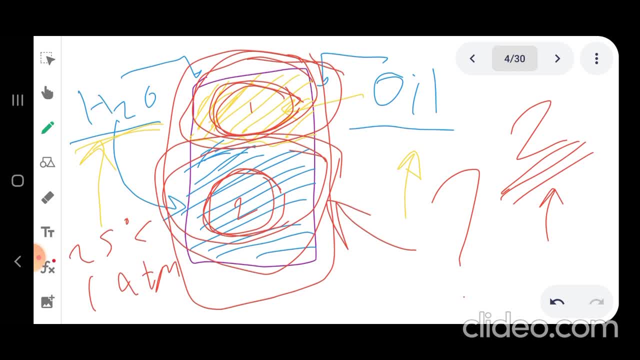 contrast and the composition, the chemical makeup. that's why we can say: in this system we have two phases, one phase is oil mainly, and the other phase is H2O mainly- okay, and in between these phases we have a vase boundary or vase interface. here, in between these two phases we have a vase. 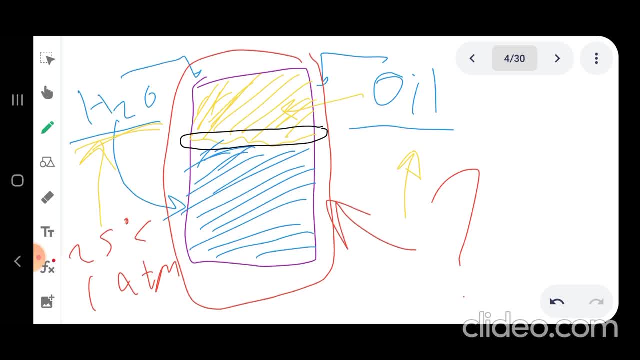 boundary. a vase boundary is something in between the two phases. this is we call vase boundary. okay, or vase interface, okay. so this is was a was a the meaning of liquid-liquid. this is how we can have two liquids that are in two different vases. in two different vases because of the contrast and composition. okay, so let's back. 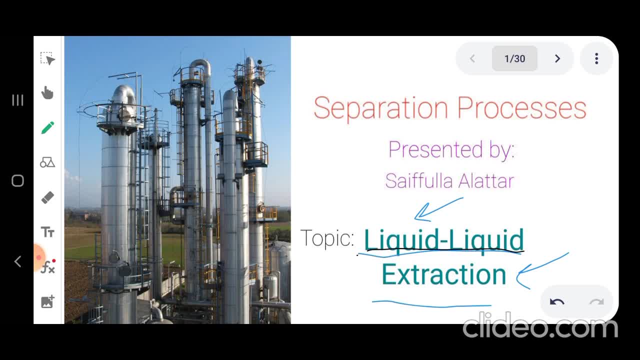 to the title, this is liquid-liquid, so we are talking only about two liquid vases, not like distillation, where we have liquid and vapor. no, here we have liquid and liquid, but both are at different bases. okay, liquid base one and liquid base two. okay, extraction: what do? 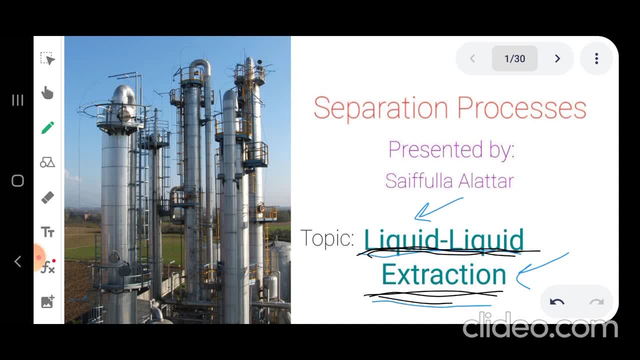 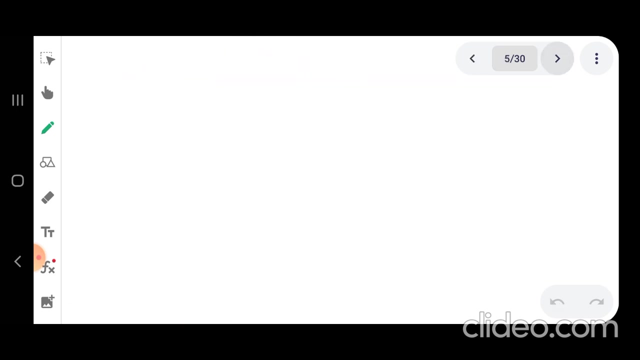 we mean by extraction? it seems like a new separation technique. it is not distillation- we finish with distillation, but now it is a new separation technique called extraction. so what do we mean by this separation technique? what do we mean by extraction? this is our topic today: extraction. in simple words, it is like when you have 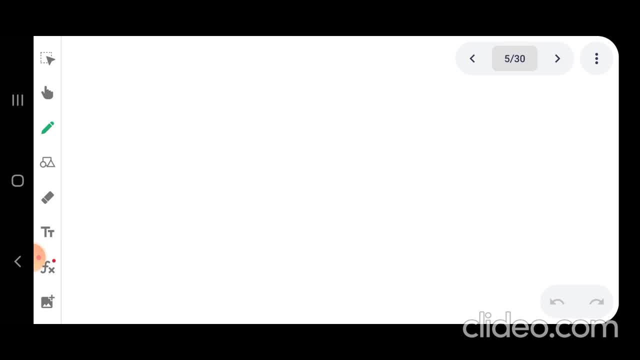 again, we are dealing only with liquid. no vapor here, only liquid extraction. it's like when you have, suppose you have- a mixture between, let's say, component a and component c. okay, let's suppose we have this mixture and we want to separate this, these two components. we 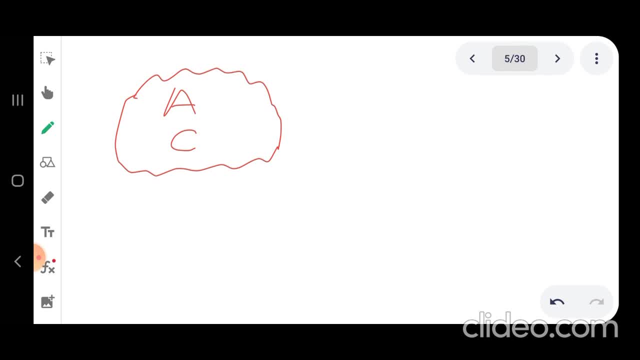 want to separate a from c. okay, so what you can do, you can take this mixture. you can take this mixture and feed it to a distillation column and get your distillate and waste stream so you can separate. it depends on which one is more volatile. so you can get this a. if it is more volatile, you can get. 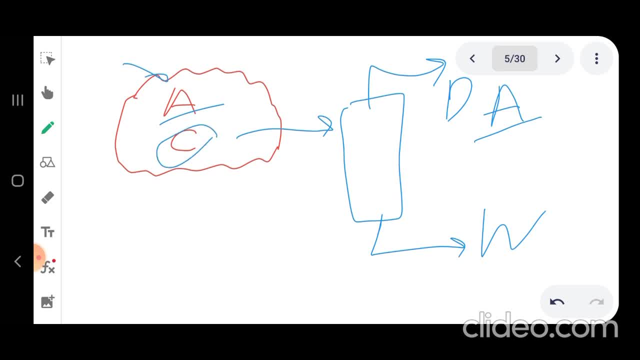 it in the distillate and you can get this c, if it is heavier, you can get it in the waste, or vice versa. it depends on the relative volatility, as we discussed before, in the distillation. okay, but the question here: what do we? why do we need extraction sometimes? why do we need? 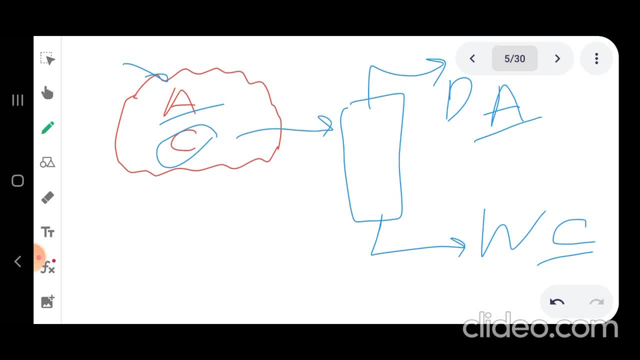 extraction. why do we feel the need to develop a new technique to separate components rather than the solution? the question here is that there are too many reasons. it's not only one reason. there are too many reasons. some of these reasons to skip distillation and go for extraction is that sometimes, sometimes you have 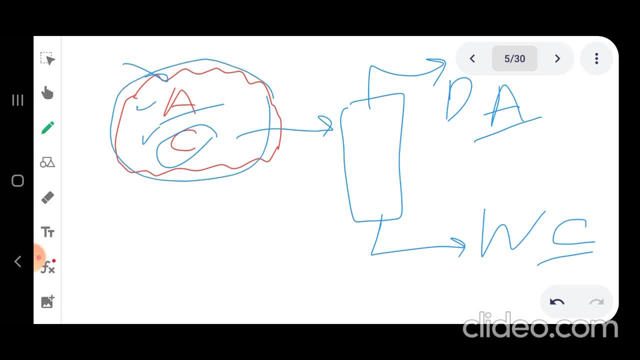 these two components, let's say a and c, they are very close in boiling point. they are very, very close in boiling point. in other words, they can form as utope and, as you know, as utope is bad for distillation because it makes it more difficult. 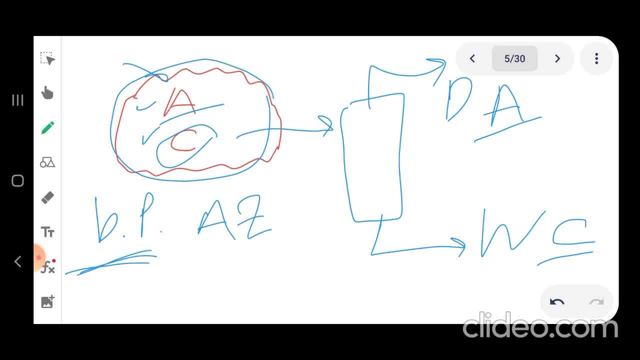 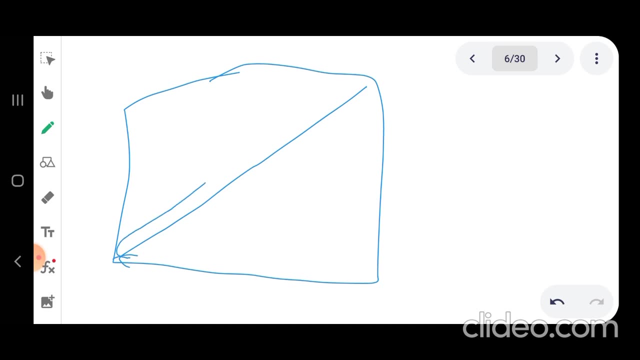 to separate these two components. to illustrate this, it is like you will get if you use makeup antenna method. you will get something like this. what you have this is the 45 degree line. you will get a tight equilibrium curve, very tight. that's very close to the 45. why? because this equilibrium curve. 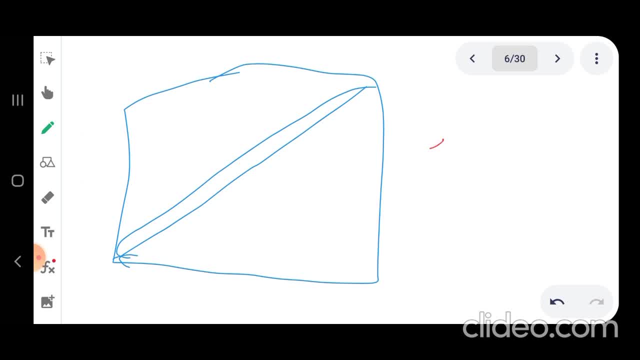 as the relative or, let's say, at as utope. if you have as utope, you will have very low relative volatility. that's very close to one. in other words, it's very close to the 45 degree line. okay, and as this relative volatility increase, you will get bigger and bigger. 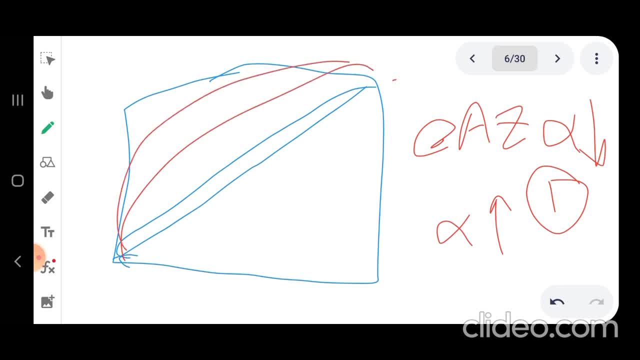 curves. okay, so let's see, let's say, in this blue curve represents a equilibrium curve for as utope. so what happens after you draw the operating lines? as we know, before we do operating lines and feed line and waku line and another operating line, so what will happen? 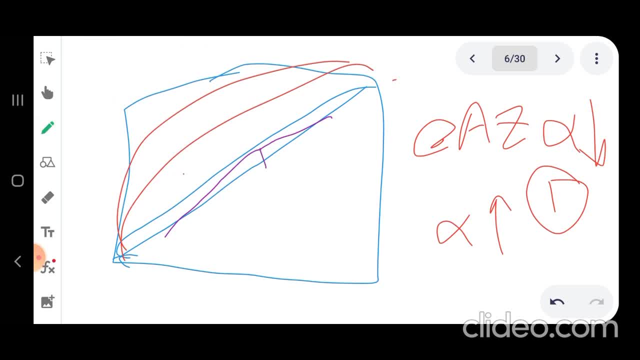 you will get too many number of stages, see, because it is tight: one, two, three, four, five, six, seven, eight, nine, very tight. then you can get, i don't know, 20, 30 trades. you need too many trades rather than suppose if you have a high relative volatility. in other words, high relative volatility means 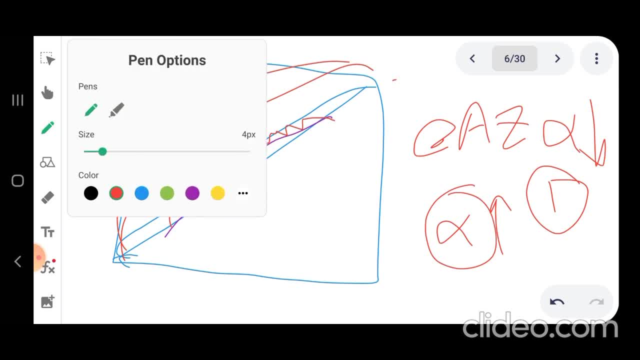 high difference in the boiling point, so you will get lower number of trades. see like focus on the scale, for example. so let's start here. we get one, two and that's it only two stages. so you can see that the higher the rate of volatility, in other words, the higher the difference in boiling point, the 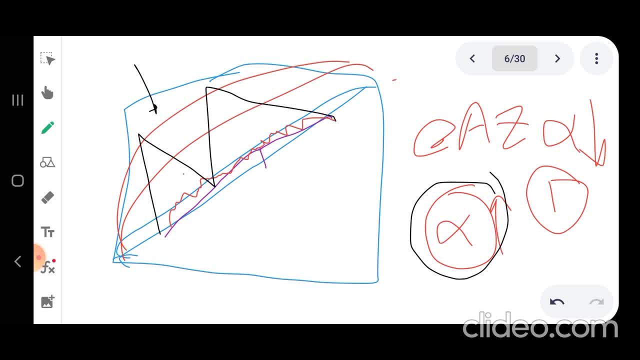 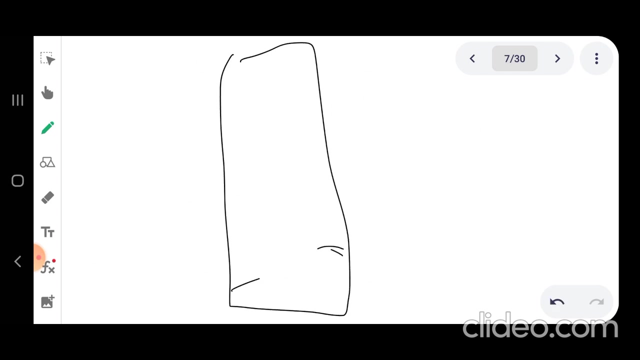 easier the separation by distillation is, and vice versa. the lower the rate of volatility, the lower the difference in the boiling point between the two components, the more difficult the separation by distillation is, because you will need too many stages. okay, you need too many states. in other words, you need very tall column. very tall column means extra money needed, so 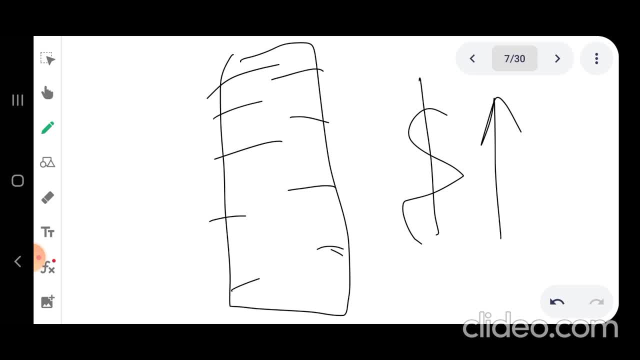 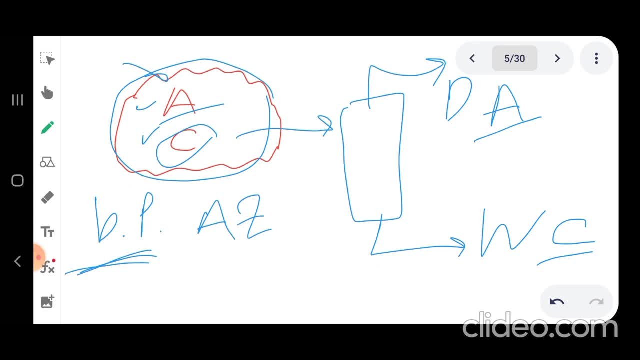 sometimes separation by distillation is not feasible. it's not good so. so this is one case where you have the two components are very close in boiling point. for the example, one of these components boil at 45 degrees c and the other boil at 48 degrees c boiling point. 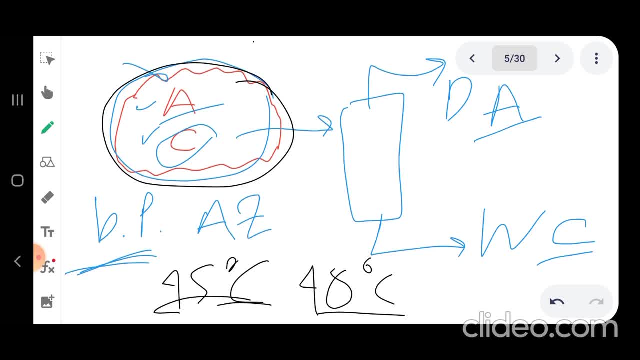 these are very close, so separation by distillation looks to be not feasible. okay, another situation, another reason, for example, is remember, in distillation we need what we need: a reboiler here, a reboiler when you heat and then get this coil up back to your column. you need this reboiler and 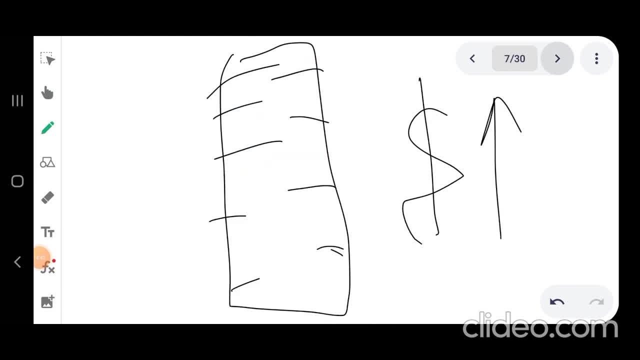 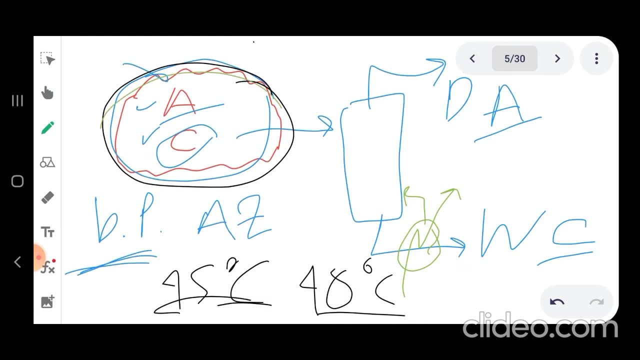 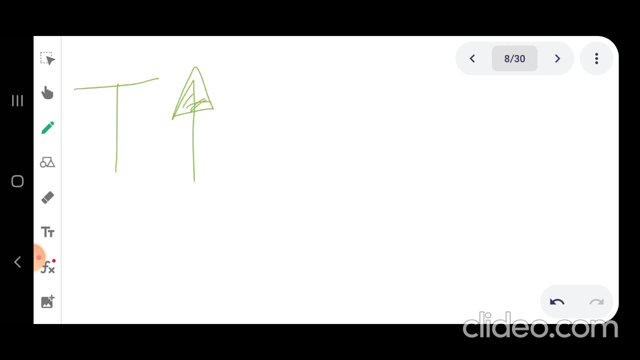 as you know, this reboiler will increase what? this reboiler will increase temperature. okay, this reboiler will increase the temperature. what happens? some components, for example, let's say our components here in this example a and c, these components sometimes what happens? at high temperature you initiate other chemical reactions. so, for example, at this high temperature, 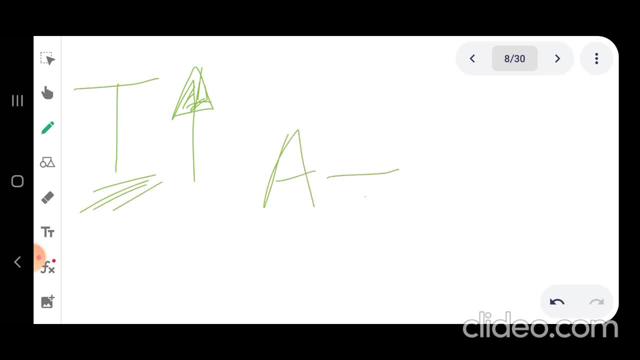 of the reboiler, a will react with c to form another component- i don't know, for example, d, just as a name. so, and this reaction only activated at this high temperature. so this is bad. you are losing your components, you are losing your components and you are. 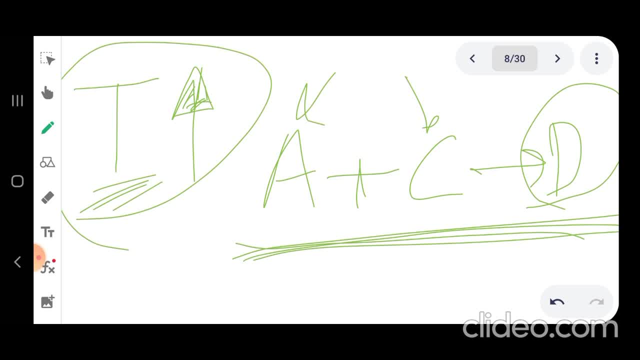 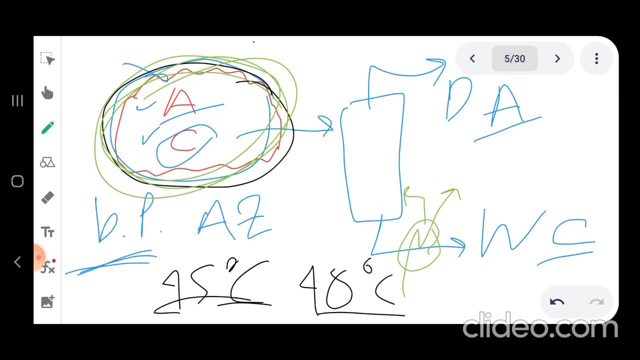 just stopping to form this third component, that maybe you don't need it, you don't want it. so, in this case, separation by distillation is not good. separation by distillation is not good and you need to look for an alternative process. okay, so this is just an example. 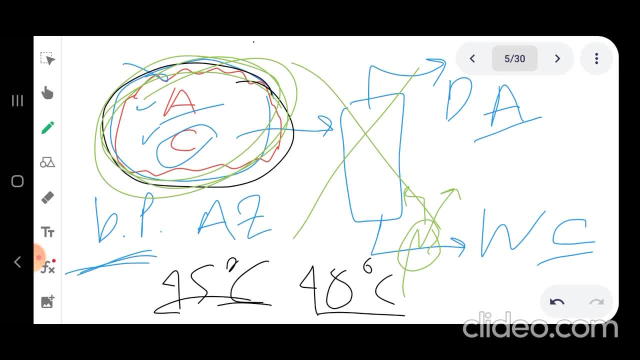 of typical reasons to go for this, to go for another separation technique rather than the most fundamental famous separation technique, technique which is distillation, okay, okay. so one of these alternatives that we can go for is extraction. we can go for extraction, especially if you have liquid base, liquid liquid extraction. so again, big the question here: what's the? 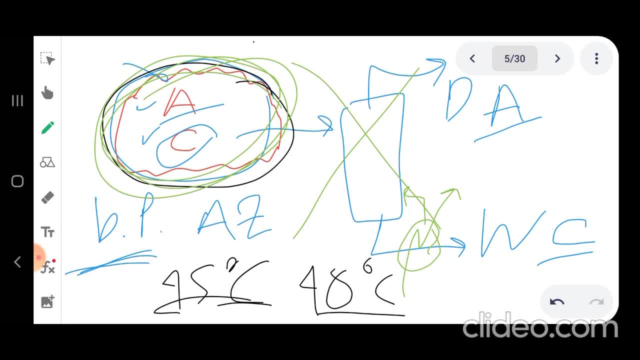 meaning of extraction? what's the meaning of extraction? as you might think, the first thing that may come to your mind is that in extraction, we don't need a reboiler. okay, why? because we say it and sometimes we avoid distillation because of this reboiler that has a high temperature that initiate another 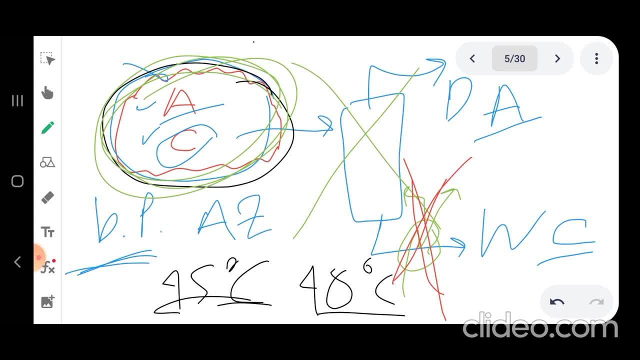 chemical reactions. okay, so this is one thing that comes in your mind. the other thing that may come to your mind is that separation by extraction is independent on boiling point. it does not depend on the difference in boiling point. so it is not like this distillation. it's a different separation technique. okay, no matter it. 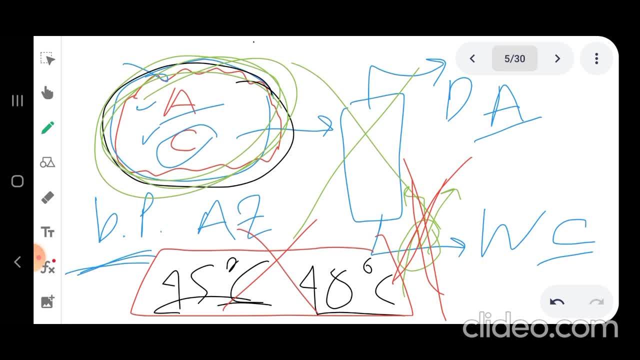 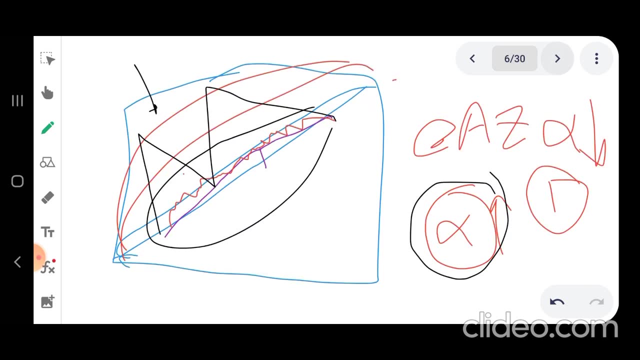 doesn't matter whether you have a close boiling point components or when they are far away from each other in boiling point, so it doesn't matter, okay. so again, what's it? what extraction is extraction? simply in a simple words, it is like when you have, suppose you have again this mixture that 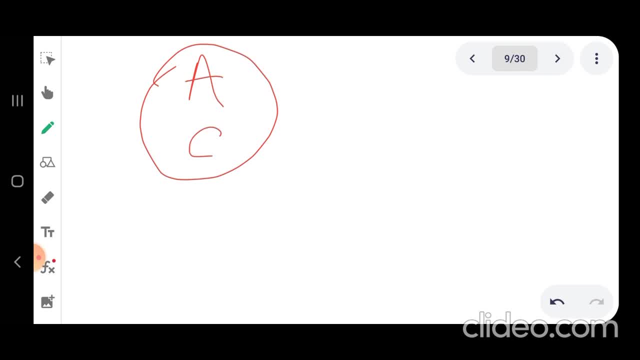 consists of A and C. okay, so what you do? you mix, you mix this mixture, you mix this mixture with a solvent. a solvent, let's say this solvent, let's call it B, for example, let's call it B. so you mix this mixture. you want to separate for. 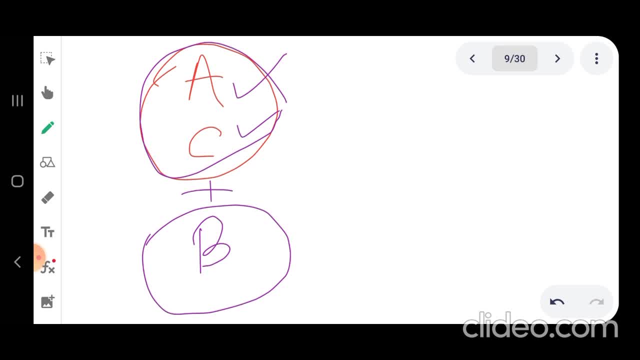 example A from C. so what you do, what you do, you take this mixture A and C and mix it with the solvent B. okay, but this solvent has some conditions, some restrictions. the first thing, suppose suppose you want to separate this A, you want to take this A out, you want to separate it, okay. so you need to choose a. 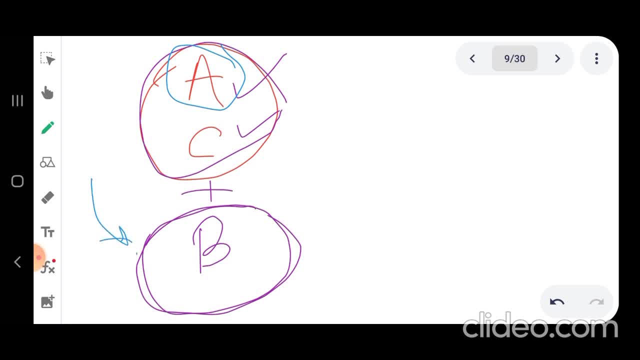 solvent that somehow chemically attract, attract this A and, to some degree, do not attract this C. okay, to better illustrate the concept, let's back to our example of oil and water. okay, let's back to our example. what do you think which is easier to dissolve in? 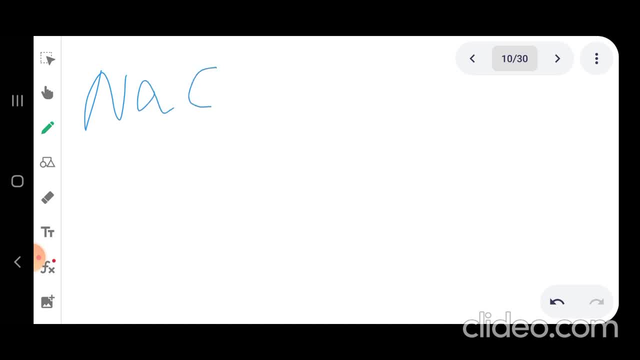 NaCl. NaCl, which is salt in water or in oil. what do you think which one is easier? of course, to dissolve it in water. okay, so you make this salty water like sea water. sea water is a salty water, right, okay so, but is it easy to? 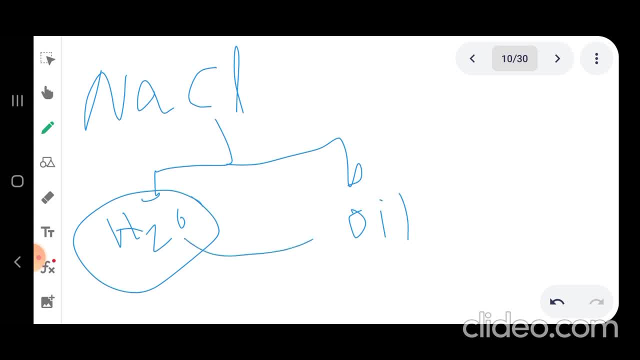 mix to dissolve H2O in oil. as we see before, it is not easy, because later you will get this layer that where you here have this water and there you have l oil. okay, so we can say that we can see that water dissolved in Acl easy, okay. so 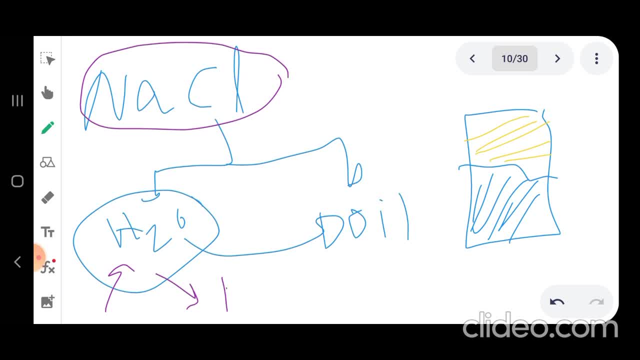 we can call this water b-sulfate, for example. okay, and the solute which, which is NaCl, we can call it A and let's call Orion, for example, C. so now suppose you have a mixture of NaCl and Orion. you have again. this is A and C. as we said, A represent NaCl. 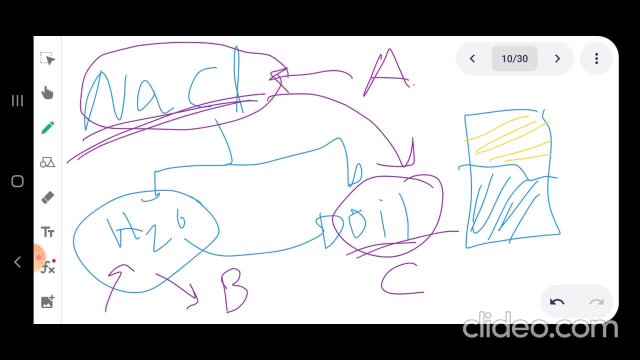 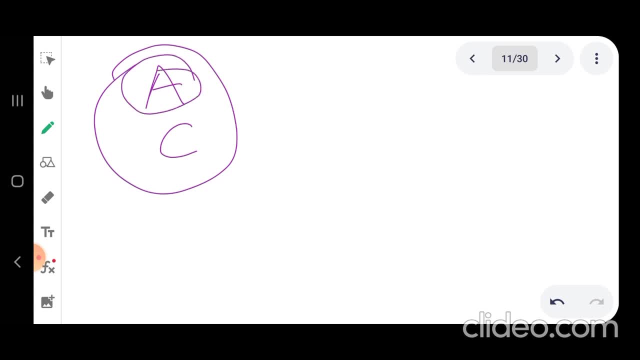 salt C represent oil. okay, let's say you are interested to take this A, which is the salt, out. you want to separate it. so what you will do, you can mix it with water, H2O water, which is B. we give it a symbol B, so this water, which is the solvent, will chemically attract this. 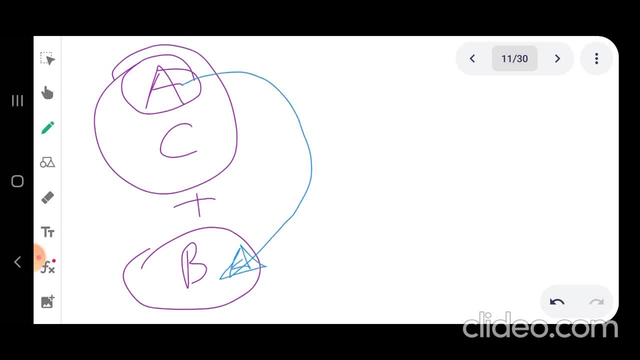 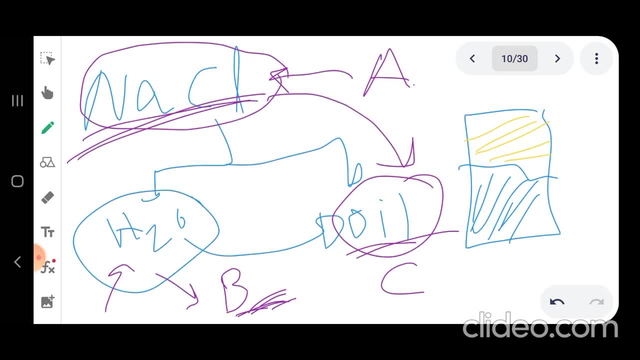 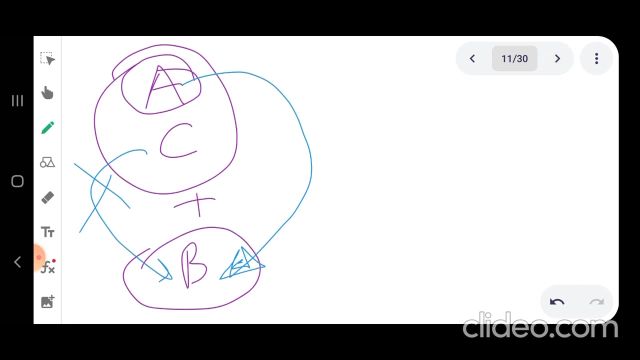 A and will not attract C, why, and as we said, oil and water usually form these two phases, they do not mix. after some time, you allow some time for the equilibrium to be rich, you will get two phases of oil and water, okay. so what happens after you mix this two? B will take this A. B and A now come together. 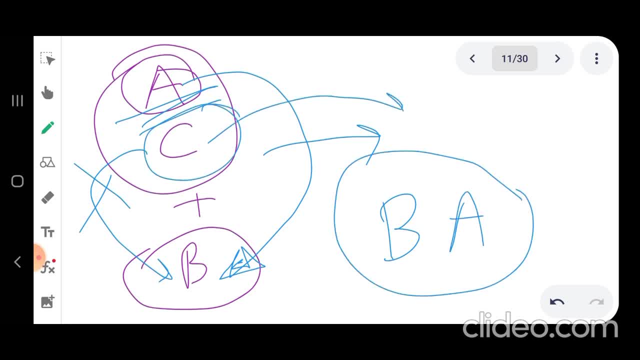 and then you left with this C. okay, to some degree, it is not 100%. yeah, for example, you can have I don't know 0.1% for example, A here and B there, but mainly you have C and mainly you have mostly most of the A is attracted by the solvent B. okay, which? 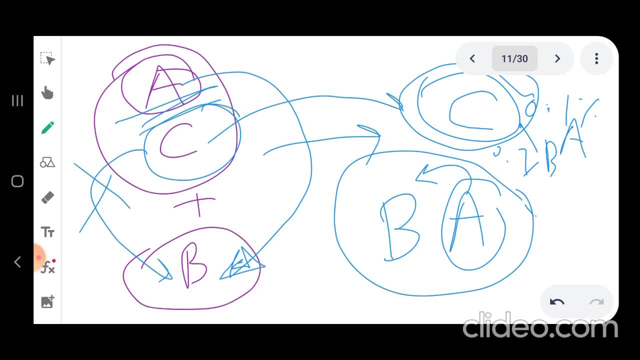 is now good. separation is achieved. you separate a from C, so you have this almost pure C- it's not 100%, if you see, but almost pure C- and the rest B&A, which is another mixture that, for example, maybe it is good for distillation to separate. so you can take, for example, this: 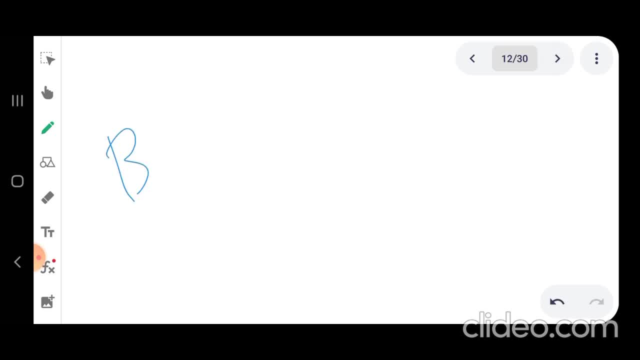 ba. you can take, for example, this ba and feed it to a distillation column and then you get your a and your b, for example by distillation. so maybe this mixture is better to separate by distillation. so it's like steps. usually extraction is not alone. usually you have this extraction and then you have. 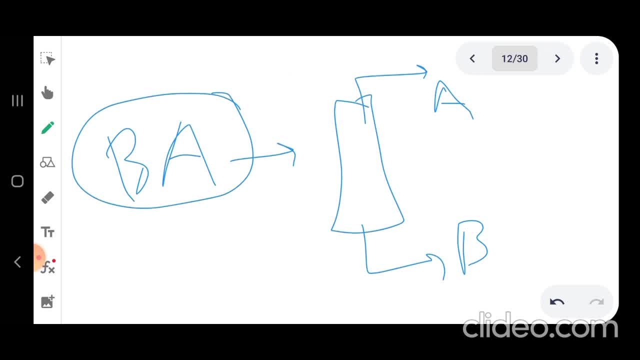 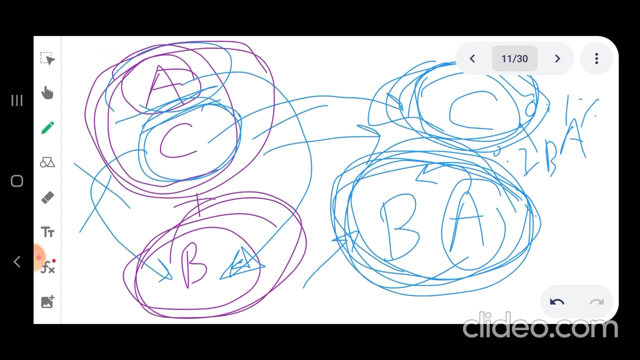 distillation. okay then, what you do, you can, you can take. you can take this b, which is your solvent, back, recycle, recycle it back. you can take it back and recycle and use it again and again with a new feed of a and c. then b takes this a and then you take b, a feed to distillation. you separate. 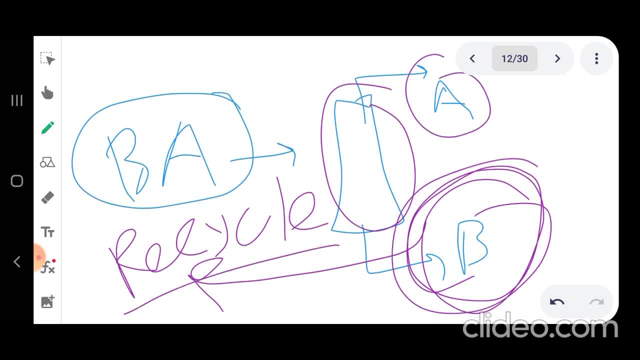 a from the solution, so it will. one goes here, then you do this, so you know that you have distracted. all the distillation specificic IC间 overwhelms your prepared surface area and you were first there B and then the circuit B and use it again and again. so this is how things go. 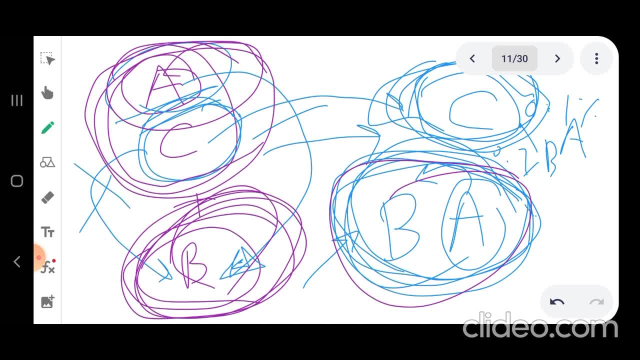 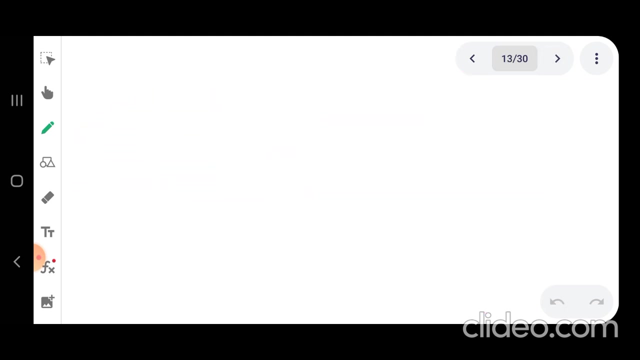 in real industry. but again, our focus here is only on extraction. in this chapter, we are going to focus only on this step, on this step, which is extraction. so how extraction takes place. this is our focus in this chapter. okay, so, before we move on, before we move on. 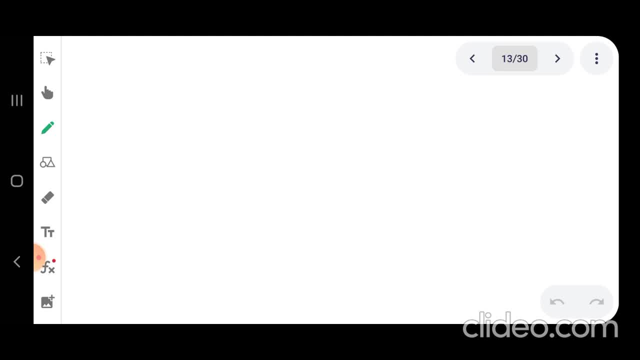 let's find first agree on the symbols. let's first agree on the symbols. so let's say components and extraction. we have three components. we have three components. it's not like distillation, if you remember, in distillation, when we talk about distillation, we can have binary mixture or we can 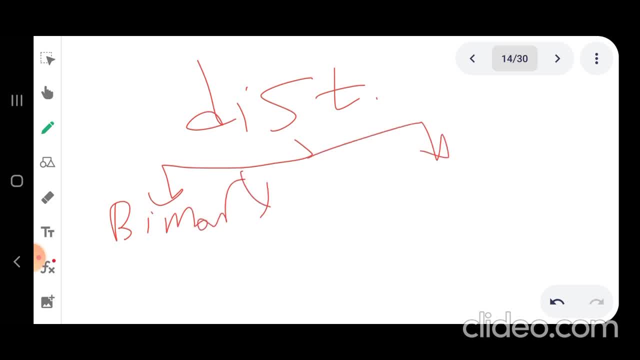 we can have multi-component mixture, multi-component right and, as we said before, for binary mixture we can use make-up delay method or function separate method to analyze the distillation column in multi-stage, in not multi-stage, sorry- in multi-component we can rely on. we cannot. 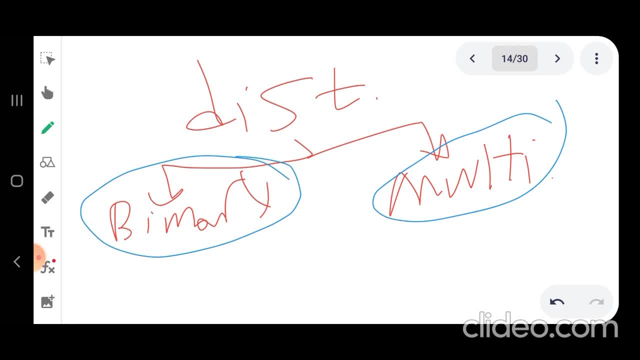 rely on graphical solution, we can rely on approximate solution like Fug matrix. we can method Wienerski-Underwood-Geliland correlations or, if it is single, for multi-stage distillation, and if it is single stage distillation, we can use that Rochefort-Reyes equation to: yeah, and that's what we have talked about. 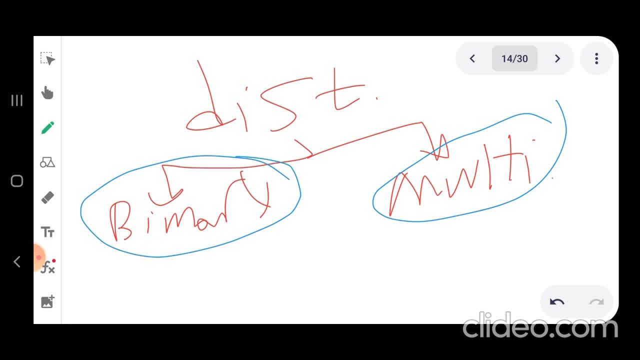 before, but now the story is different. when it comes to extraction, mainly for simplicity, we are going to focus and deal with three components. three components so it is not binary system where you have A and B. in distillation, binary you have A and B. no, here in extraction you have three components in. 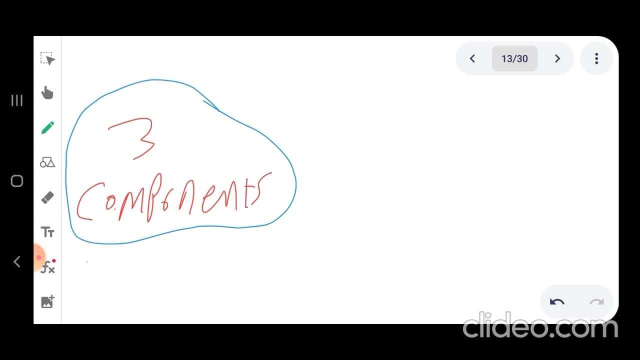 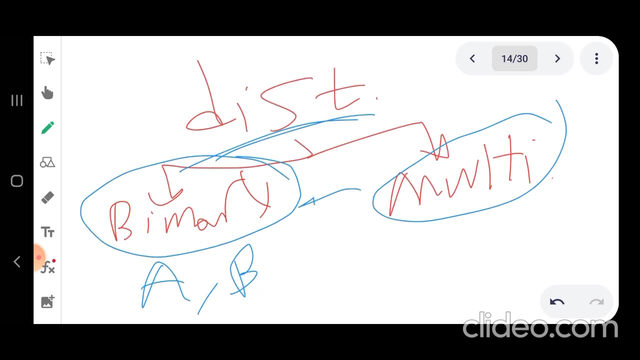 other words, we call it ternary system, not binary ternary ternary system. you have this ternary system. what do mean by ternary? ternary means three. it is like binary binary means two, ternary means three. so we are going to deal with the three components, so let's give them a. 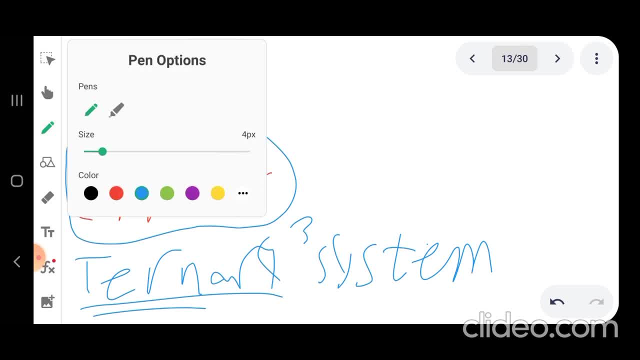 simple. just to agree on the simple, to not confuse you later. so let's agree from the beginning on the simple. okay, so let's go back to our example, which is oil, NaCl, salt and H2O water. so, as we said before, in this case NaCl is the solute and H2O is a solvent. this is 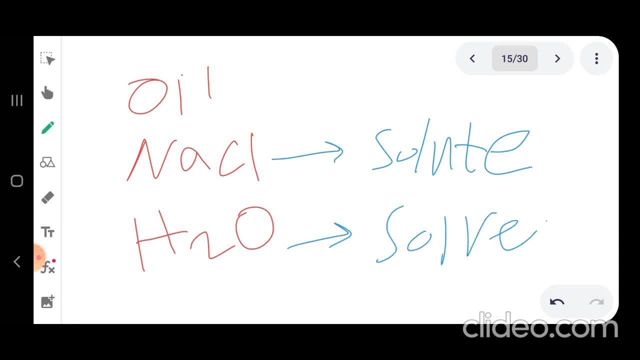 this: this is the solvent that will attract lessANT戲. it will attract it. okay, and this oil, we call it that remember. so let's again not confuse you remember, initially we have this oil and NaCl mixture, okay, then we add the solvent, which is water we added. then the result is: 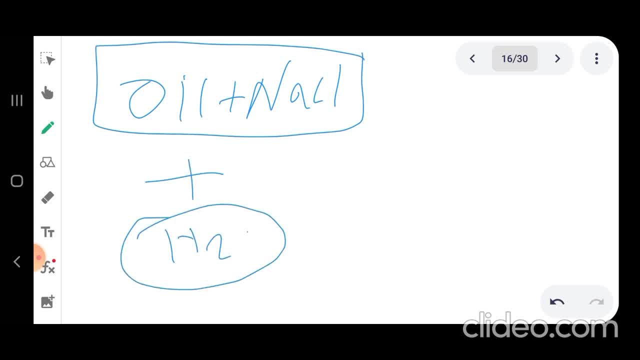 an Multiple reaction problem. لا bucks, Novice, obviously let's go ahead and try some else, but let's use another example. is that water attract, water attract this, NaCl attract the salt, and then we left with almost pure oil. okay, okay, so NaCl that to be attracted is called solute. 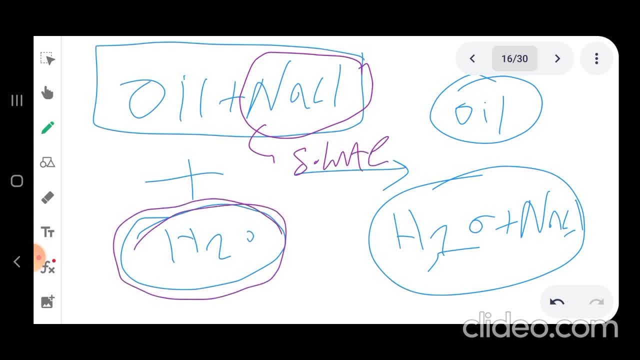 the component that will attract this solute is called the solvent. the component that holds the solute initially is called the carrier- carrier. so again, solute is to be extracted, to be taken. the solvent that will take this solute later is called solvent. so okay, so. 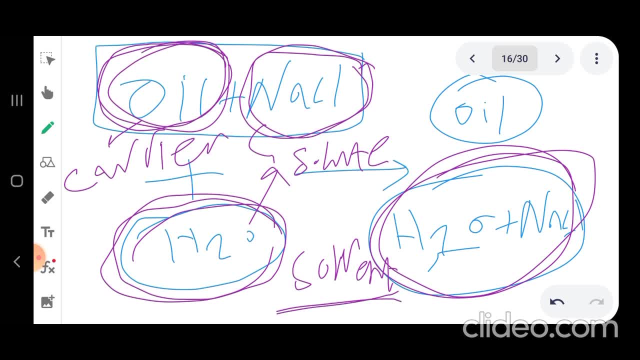 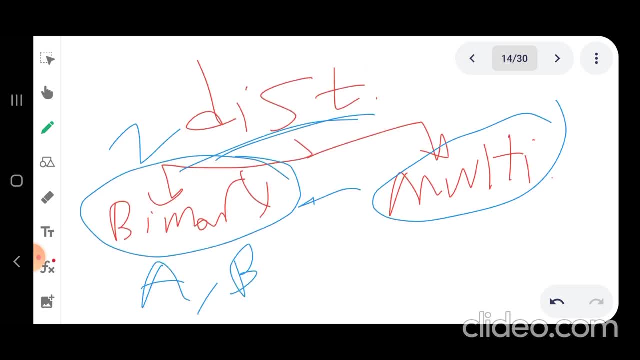 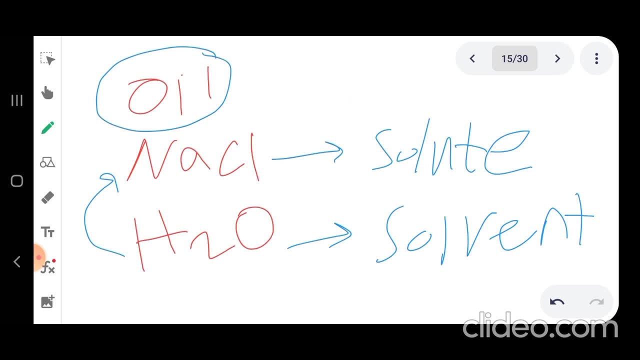 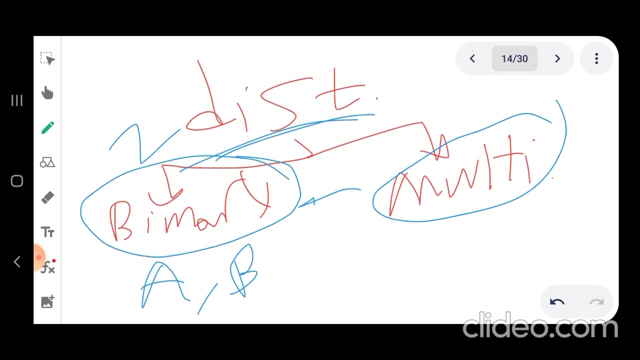 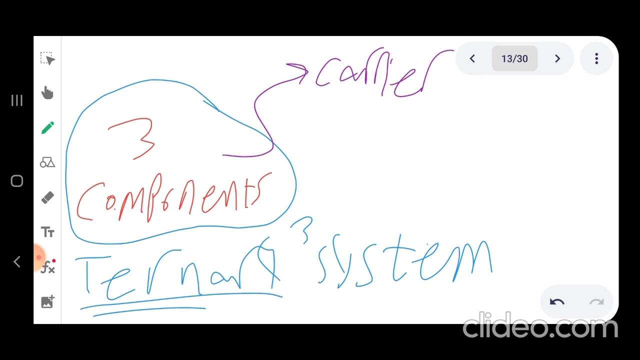 so the, the component that has the solute initially before extraction process, is called carrier. okay, so oil here in this case is considered to be the carrier. carrier from carry like play player carry carrier. okay, so let's agree on the symbols. so we have a carrier and this carrier has the solute, has the solute. 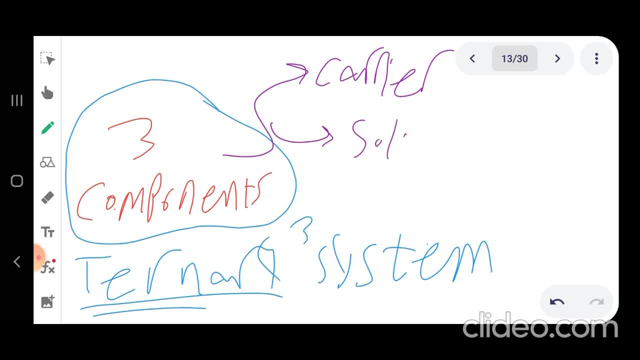 initially, and we have the solvent that will attract that solute. okay, so let's agree on the symbols. the carrier- carrier c, we are going to call it, or to give it a symbol c. the solute: we are going to give it a symbol a. the solvent: we are going to give it the 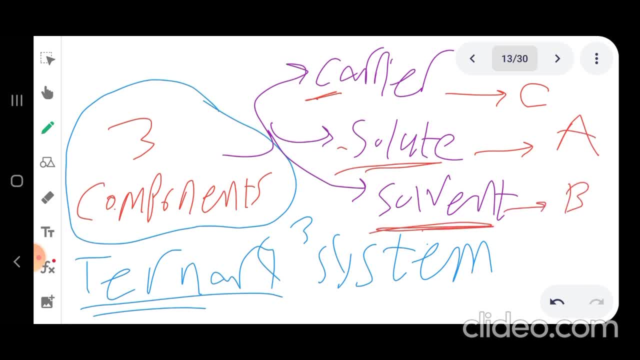 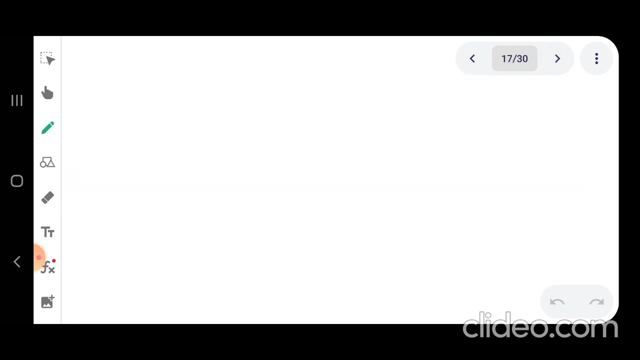 symbol b. so again, carrier c, solute a, solvent b. okay, so this is just a symbol. okay, so now let's talk more about the extraction process itself. how many types of, how many types of LLE process we have, or processes? okay, LLE refers to liquid, liquid extraction. so how many types? 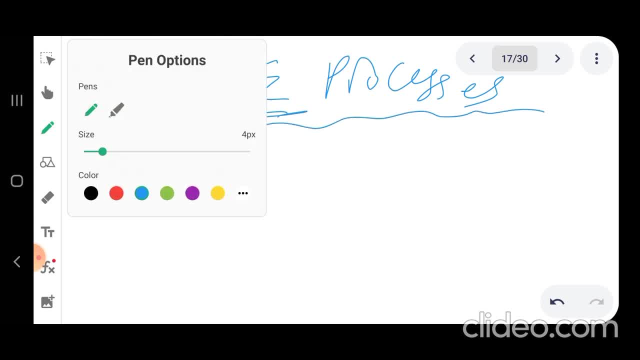 of this liquid, liquid extraction we have. we have many types. mainly we are going to focus on three types or let's say no, let's say two types, two types mainly. the first type is it's like distillation, and first type is single stage liquid liquid extraction. 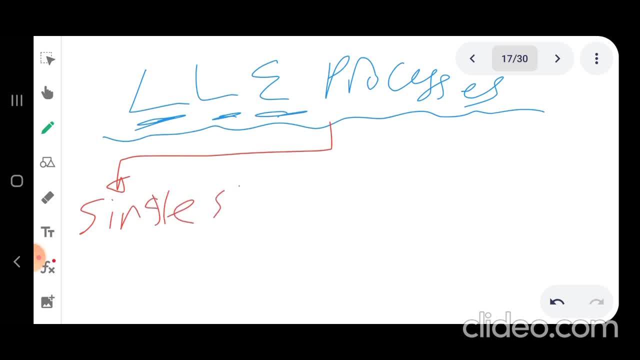 single stage. single stage extraction and the other type is multi-stage- multi-stage liquid liquid extraction. okay, and under under this category, which is multi-stage extraction, we have two subcategories, which are cross-current multi-stage liquid liquid extraction, cross current, cross-current multi-stage liquid liquid extraction and the other type. this is normal. 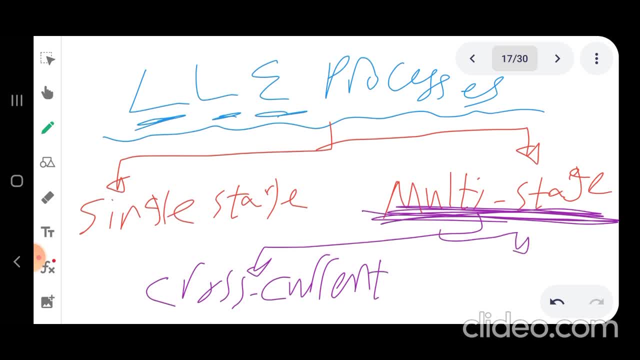 the other type is counter-current, counter-current. okay. so again, liquid liquid extraction process. we have many types. two of these types are the single stage liquid liquid extraction and multi-stage liquid liquid extraction. this multi-stage liquid liquid extraction has two modes. the first mode is cross current, cross current. the other mode is counter current, counter current. okay so. 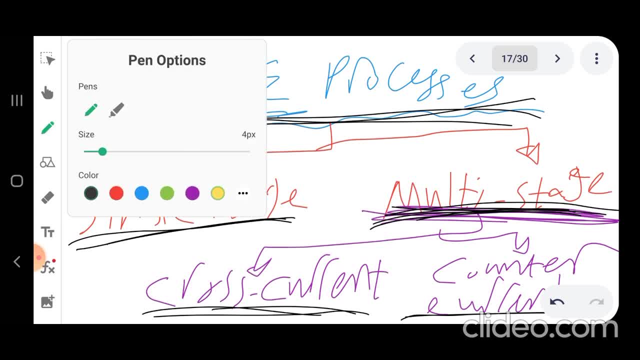 mainly we are going to spend later. the next video are going to talk about single stage, the next one is cross current and the last one is counter current. the most famous one out of this is the counter current: multi-stage liquid liquid extraction. okay, but before we go to the next video, 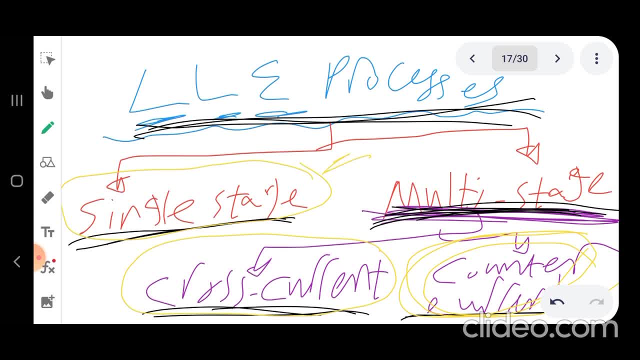 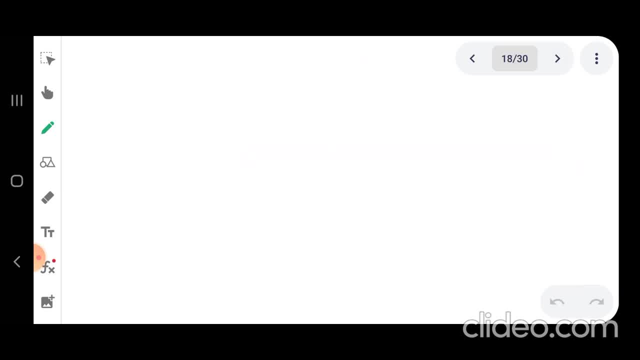 that we are going to. we are going to discuss the single stage: liquid, liquid extraction. we need to agree on some symbols. we need to agree on some symbols again, okay. so the first thing, we know that distillation is just a column. it's a column, it is a tower, a long tower. will you have the tree? but what's what's extraction? 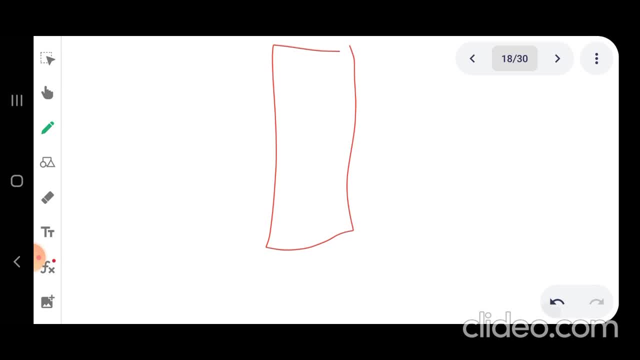 unit, extraction unit, is simply a vessel. it's a vessel. it's a simple vessel, okay, and in this vessel, if he, if it is a single stage, you have one vessel. if it is multi-stage, you have more than one vessel and that's it, equal as this multi-stage you have too. 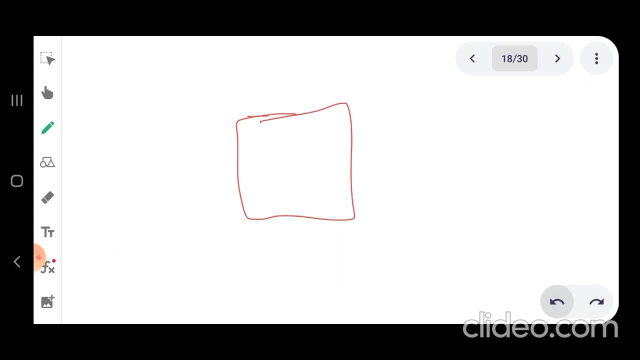 many vessels. single stage: you have one vessel, okay, so let's agree on the symbols that we are going to deal with the first thing as the feed, feed, feed, we are going to call it F, okay, the feed, we are going to call it F. and this feed, as we said before, it contains what it is like. again, we go. 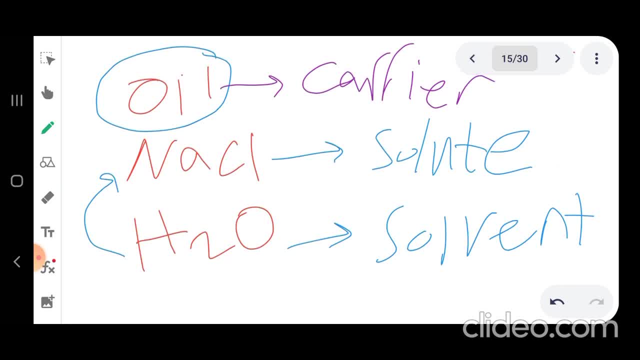 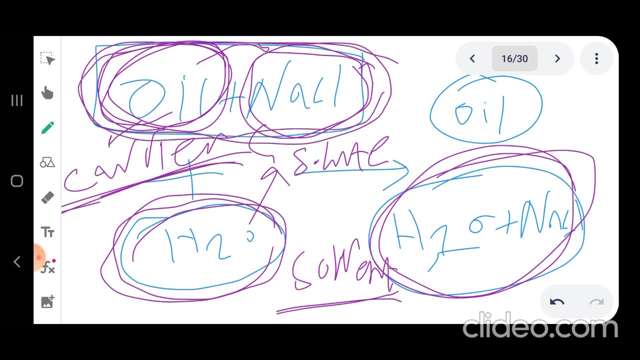 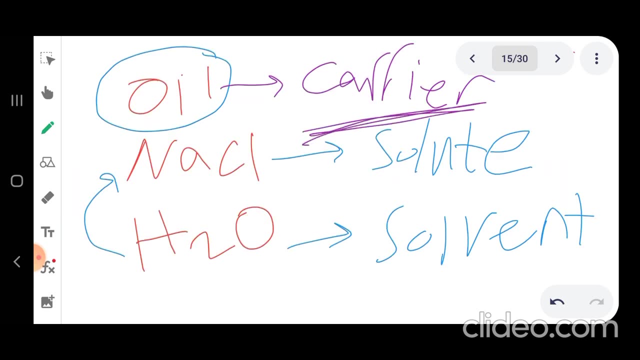 back to the example of oil, salt and H2O. so the feed contains mainly oil and NaCl or, to be more general, it contains what it contains: carrier and solute. in other words, it contains C and A, as we agreed on the samples before. so you need 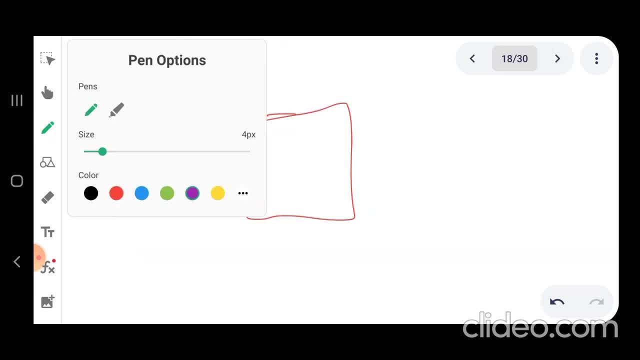 to know this by now, that the feed contains mainly a solute and carrier C. the question here: could it contain some solvent B? yes, maybe, maybe some thing times contains some of the solvent B, why not? sometimes? yeah, but it will be in very small quantities and traces and finite quantities, very small quantities. 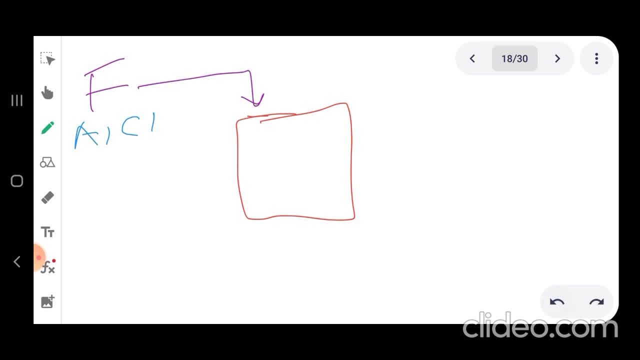 that's usually negligible, so we could have some of the solute, but mainly we will have in this feed the solute A and carrier C, okay, and then we are going to feed the solvent and the solvent, the solvent stream, we are going to call it S. I'm going to call it S. someone may wonder. 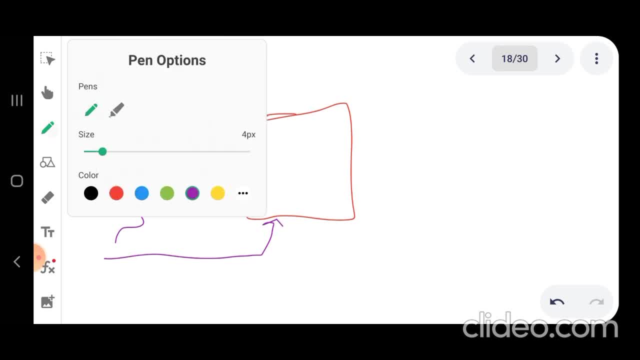 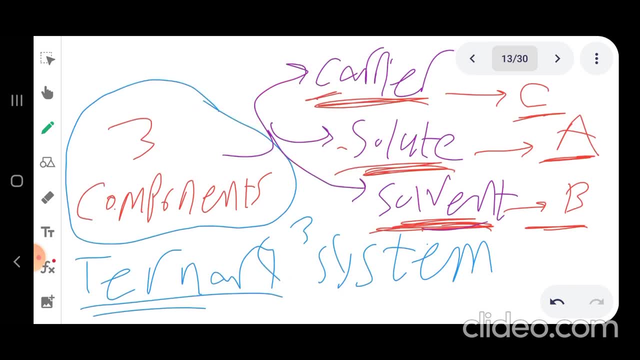 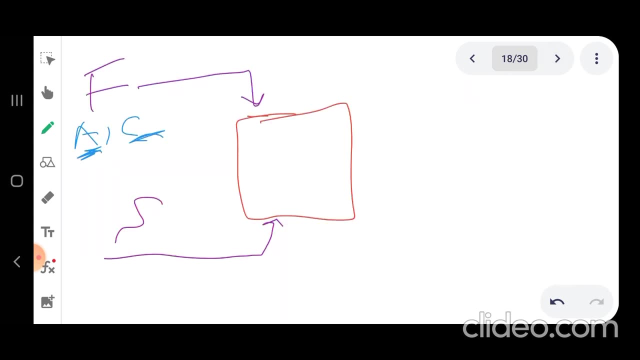 here. wait a minute. you see that solvent. we are going to call it B, and okay, so so why now you? why you call the solvent S? the answer here. you need to be careful here- why S here represents that stream. S represent that stream and this stream mainly contain the solvent B, but it 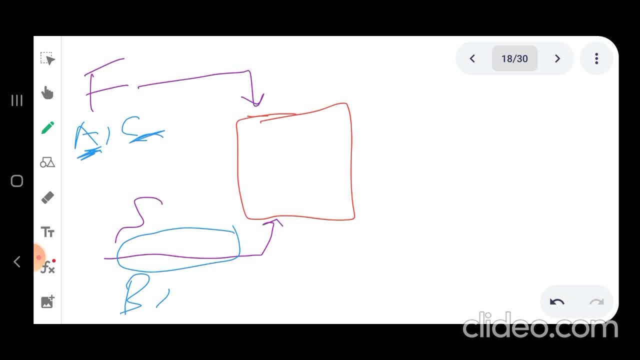 could contain some traces of the solute, or even some traces in the solute. so in which process there will be models that will not be included in this. we are coming to the last part, next moment, and I wanted to say, which is important, because it is all about adding, add HOWA JáS. 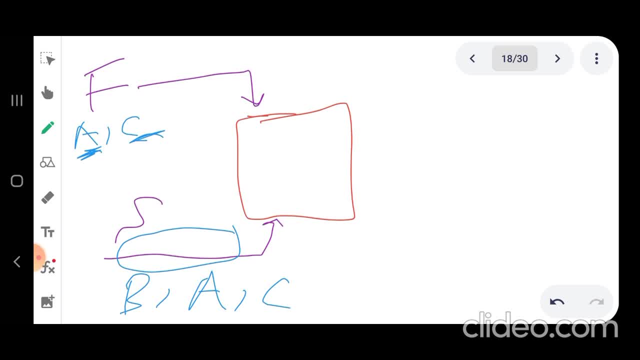 of this, the carrier, why not? okay? so again, to better illustrate the concept here, let's back to this one here, this stream. we call it feed F. but this feed is it only one component? no, we said it is mainly A and C solute and carrier. and 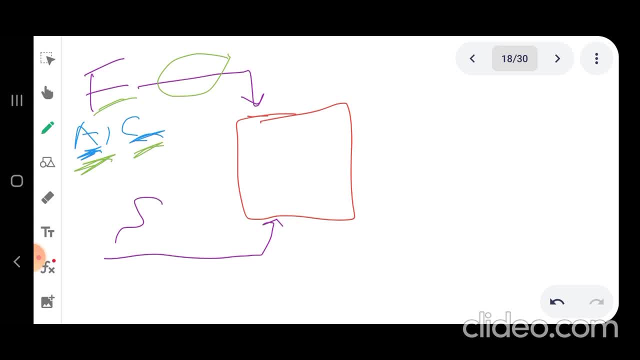 sometimes we can have some small amounts of the solvent B. okay. so you need to distinguish here between stream and component stream and component stream could contain more than one component. again, stream could contain more than one component. okay, for example, this feed stream contain mainly A and C solute and. 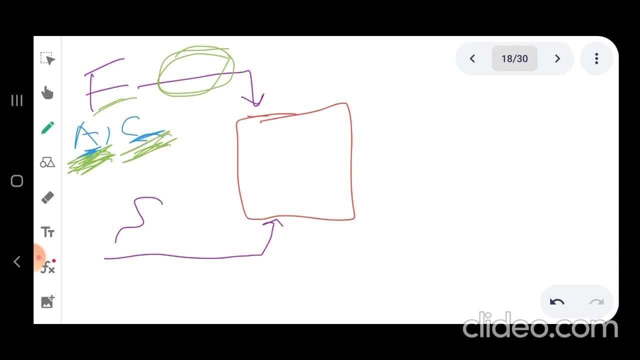 carrier. similarly, this solvent stream mainly contains B, which is the solvent, but is it always the case? no, sometimes it contains some traces or small quantities of A or even C. okay, so that's why we feel the need to call this stream as a whole stream, to call it S, but as individual components. 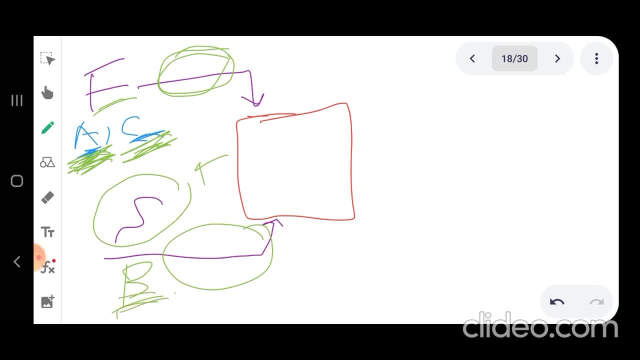 it contains more mainly the solvent component. that could be sometimes 100% B, 100 percent solvent or sometimes I don't know, for example, sometimes 99 percent B and for example, 100 percent A. it could okay, it could be the case, okay. so again, stream is different than component. one stream could contain. 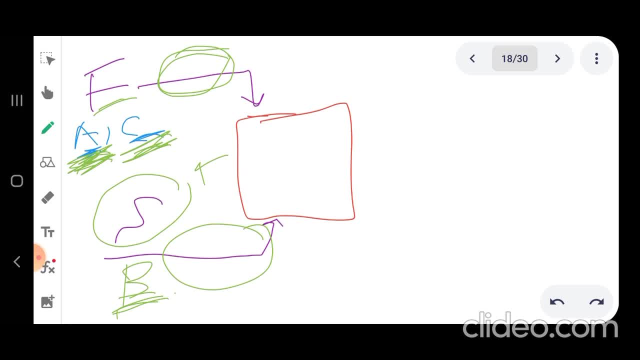 more than one component. okay, and then what happened? you mix these two together: the feed and the solvent. you mix them together so you will have inside this vessel, you will have a mixture, you will have a mixture. so let's call this mixture M, let's call this mixture M, okay, and then, after some time, you will 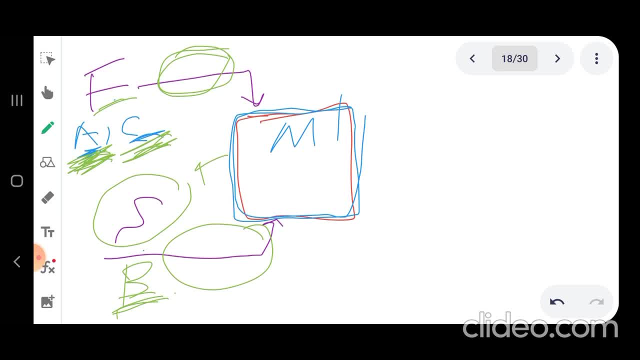 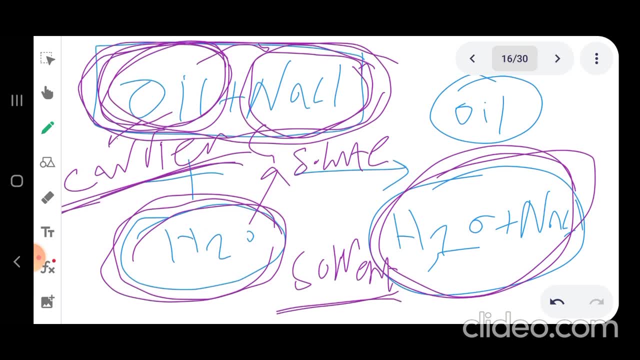 get two outlet streams, two output stream- again if we go back to the example of O nice- and h2o. h2o will attract this na Cl, so you will get h2o and H2O, these components, next command line and two 황자 helpers. and in general, this H2O doesn't actuallyl王 always grams alt iv A plus H2O oil. YES, a good point. outro, like you mentioned, peanut擊 好 haste, so you will get it: H2O and H2O. 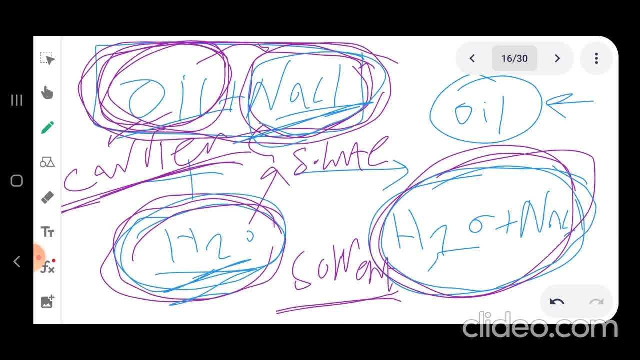 H2O- We thought it hutip also called H2O in biting H2O. so you will dig our. there's nothing in acl and mainly oil alone. okay, so in other words, what happens? solid attack, the solute and then you lift with the carrier. 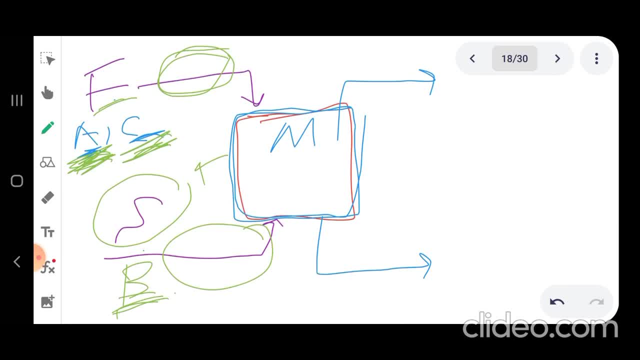 uh, sometimes we call the carrier the raffinate. yeah, we call it raffinate stream. so this, uh, this raffinate stream we will call it. let's say, this one is the raffinate stream, so we will give it a simple r. we will give it a simple r and the other stream. 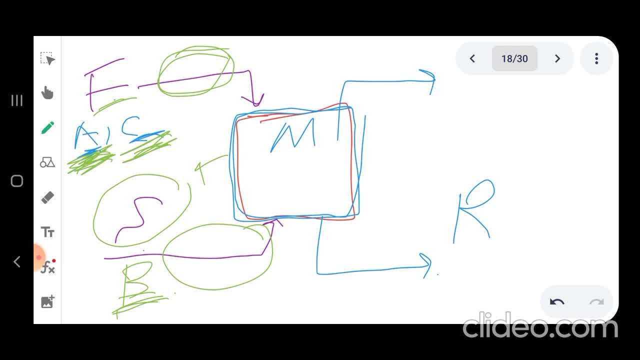 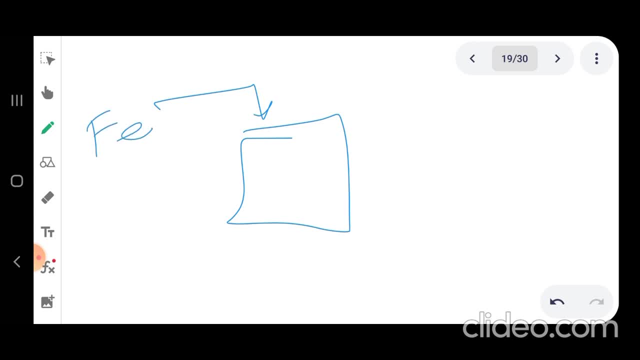 we will call it extract. so to better illustrate the concept, we have this visual. we have feed, feed stream, and we have solvent stream. then we have the output as extract stream and raffinate. raffinate stream again. this feed contains mainly solute and carrier, in other words a and c. this solvent contains mainly b. 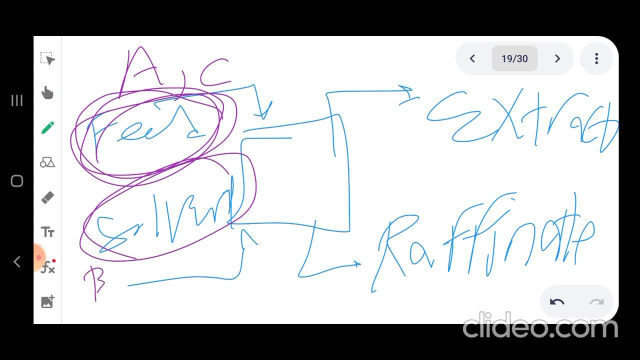 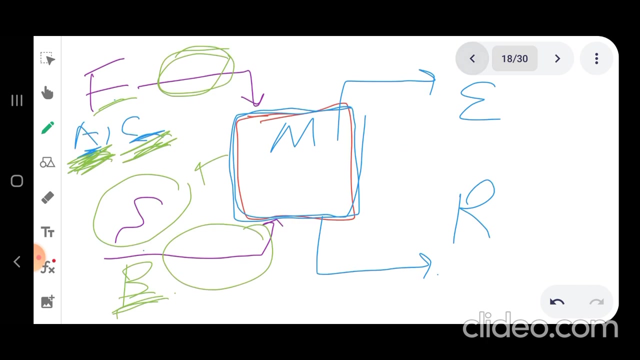 mainly b and it could be some finite, small quantities of the other components. and then this extract. what happens? this b will attract the solvent a, so this extract contains mainly a and b, okay. and then this raffinate contains mainly c, the carrier- okay. so we can go back here and say that this extract 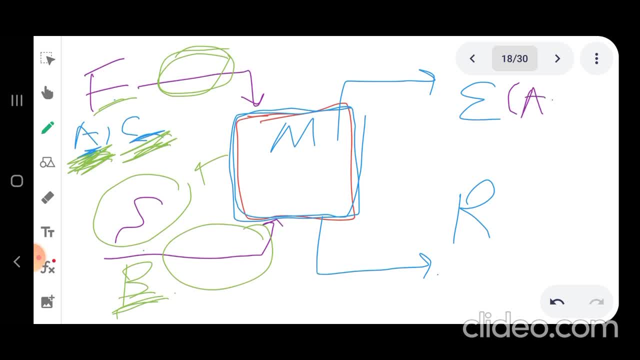 contains mainly a and a and b, solute and solvent. and this raffinate contains mainly c, but again, sometimes it's not only c. it could be the case, for example, 98 percent c and i don't know, for example, two percent b or two percent a. okay, but mainly it is. 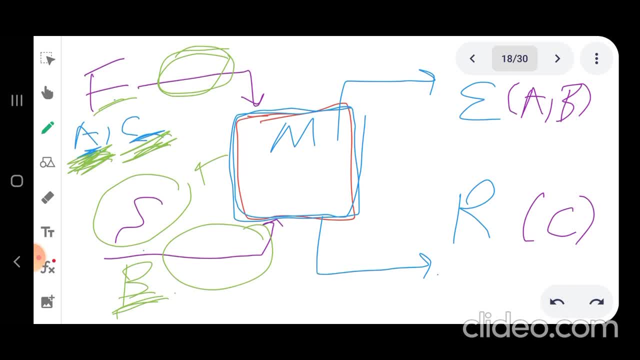 c, mainly it is c. so, as we said before, e extract is a stream, a and b are components. again, r is stream, but c is a component that mainly composed of raffinate, mainly composed of the component c, the carrier. yeah, so that's it. now let's give some. 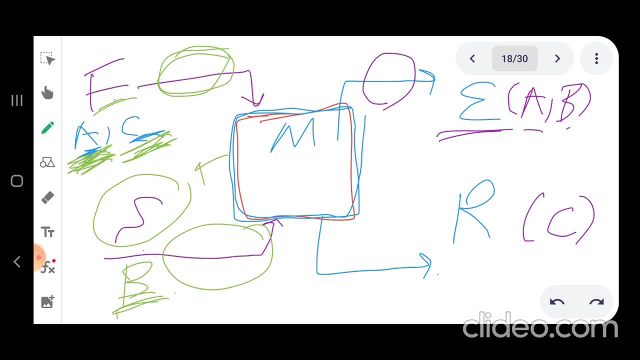 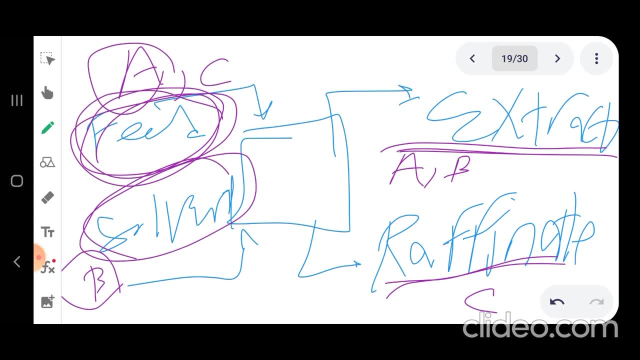 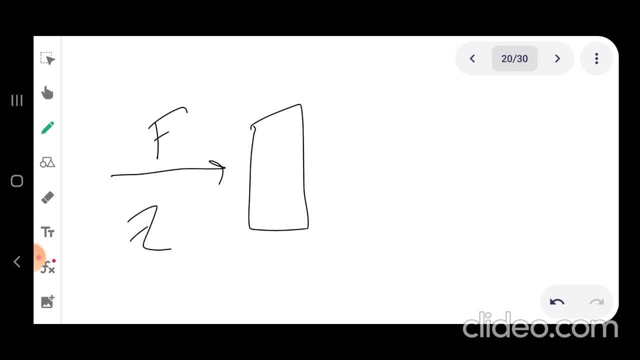 samples for what? let's give some samples for the composition. it is like, let me remind you, with distillation we said: here we have a feed and we have the composition zf, and then we have the distillate with the composition xd and then we have a waste with the composition. 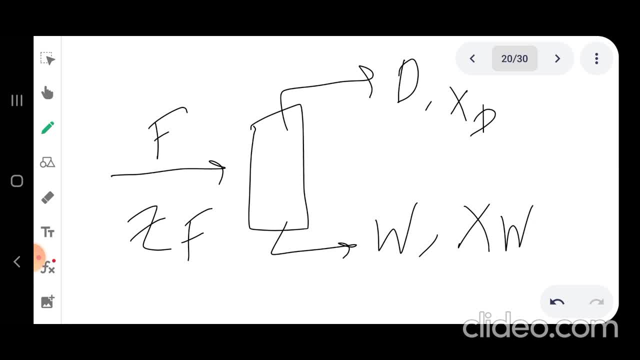 xw and, as you know, this composition of the feed or composition of the distillate, composition of the waste are, for which one, let's say the feed, is a binary mixture of a and b. so, as we said before, mainly we are going to refer all of this composition by default to the more volatile component, which is 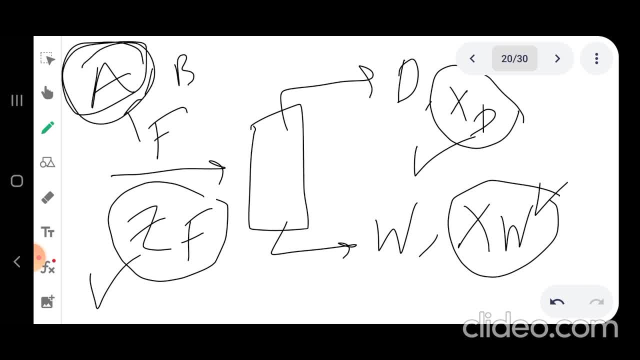 a. so when we say zf, we mean here composition of a when we make, when it's composition of a in feed stream. and again when we say xd, we mean the composition of a on the district stream. again, when we say xw, we mean the composition of component a in the waste stream. so 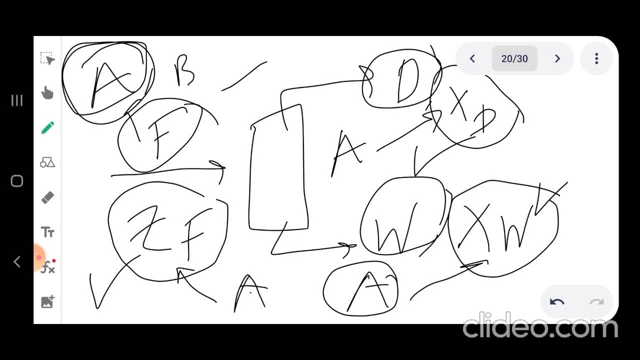 again, f: feed the stream. a is a component z. f is a composition of a on the feed stream. again, d is stream a is a component. xd is the composition of this a on that stream which is distillate, distillate, yeah, uh, I've put a row. 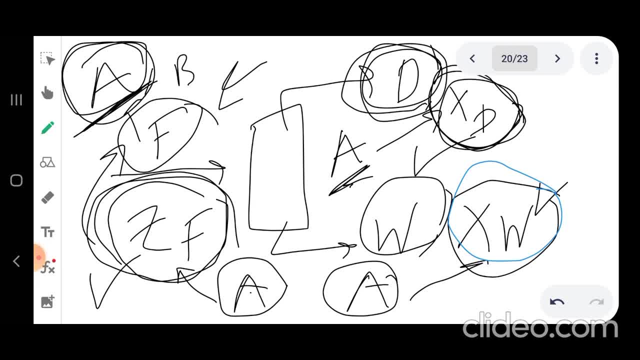 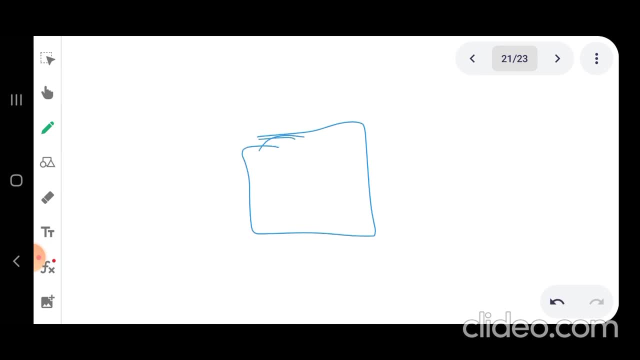 and again, XW is composition of a, which is a component in a stream, W, which is a string. okay, so we can write a quick or we can draw quick drawing again for extraction process. so for extraction process we have what we have here. this is the feed with composition of a, X feed, and we have here solvent S with a. 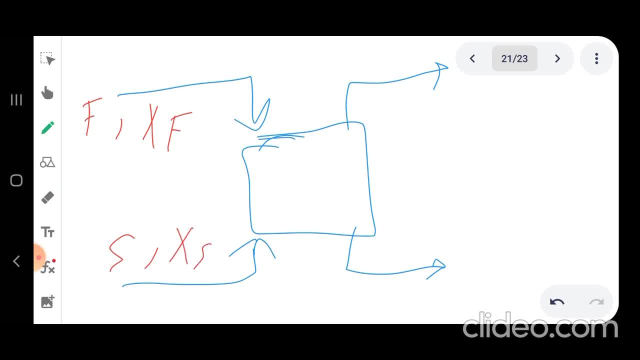 composition XS. then we get mixed. we have a mixture here with a composition XM of solute a. then we have two products, top products, which is it doesn't have also to be top product, but just for convenience we are going to do it as a top stream. 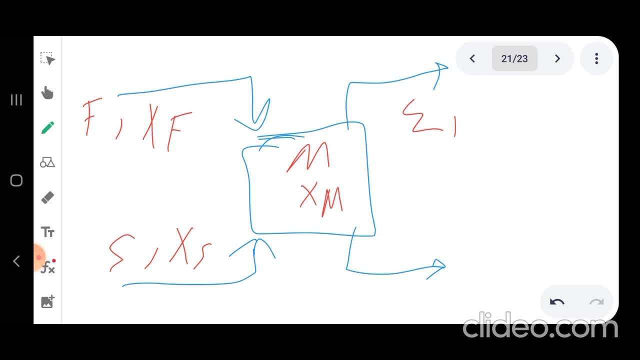 so here, extract e, well, composition of extract, XE. and then we got a raffinate R with a composition, XR. all of this composition refer it back to solute a. okay, solute a, this composition and this one, XF, XS, XE, XR, all are for solute a. so XF is composition of solute A. 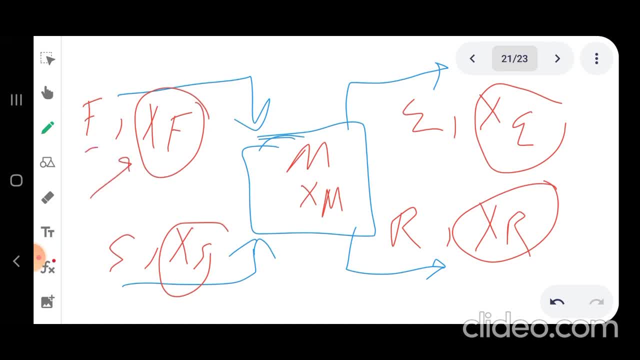 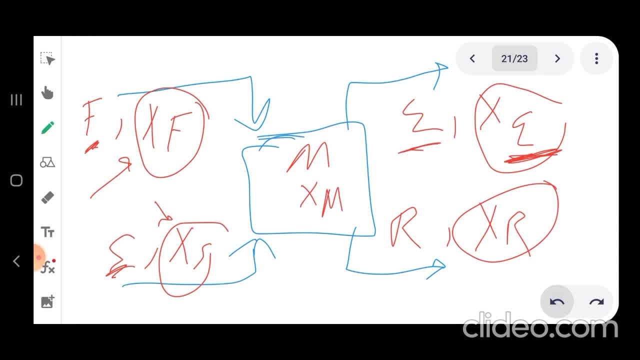 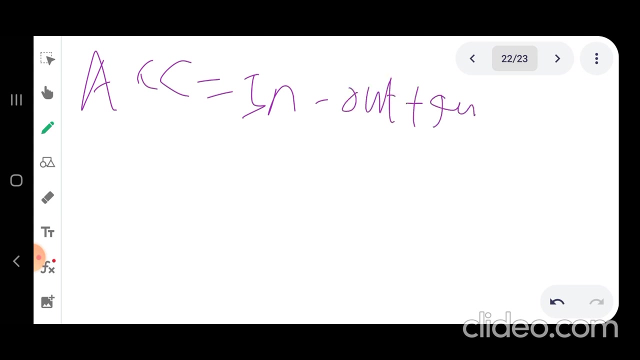 solute a and raffinate stream. okay, so now we can perform a material balance that we are going to need it later. so let's look at the overall system and then write material balance. we know that accumulation is equal to input minus output, plus generation minus consumption, and we don't have chemical reaction here, so they 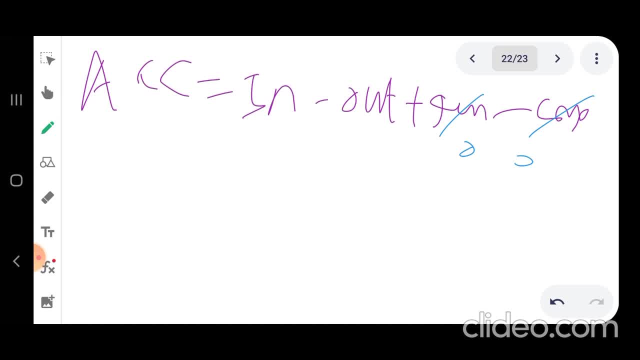 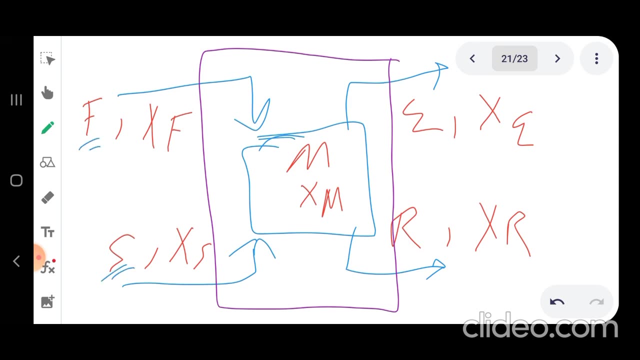 are zero generation and consumption and they assume a steady state process, so accumulation is zero. so you end up with n equal to out. okay, so let's look at the overall system. so what's the inlet and outlet? we have two inlet, f and s, and two outlets, which are e and r. this could be molar. 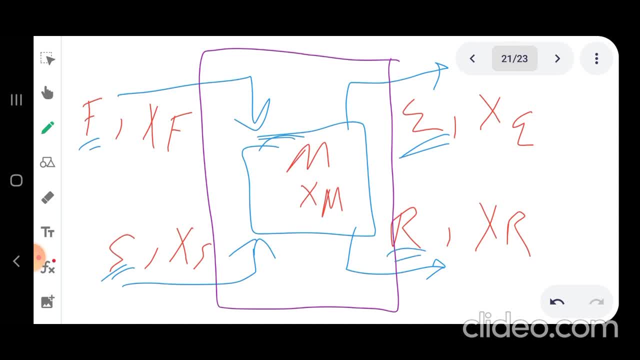 flow rates or mass flow rates. what? usually when we deal with extraction, we prefer to deal with mass flow rates usually, but it does mean that you are not going to deal with the with the molar flow rate, but it is usually. you deal with mass flow rates in extraction. so let's do this in equal to out. so 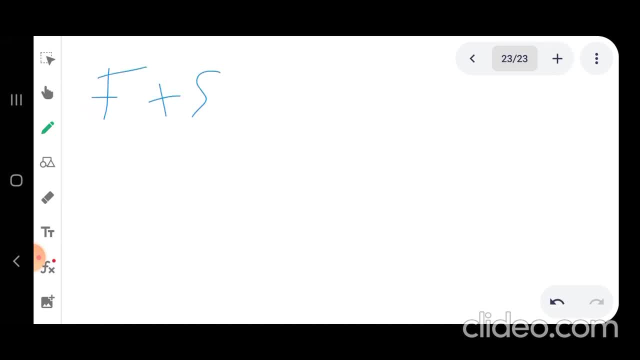 f plus s, equal e plus r. and if you want to do component, so this is overall material balance. now, if you would like to do a component material balance on component a, for example, which is our focus, so you, so this simply will be x f, f plus x s s. this is x s equal to x e, e plus x r r. okay, so that's it. 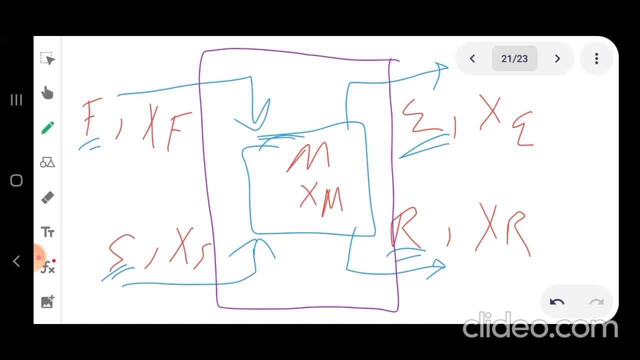 this is material balance on the overall system. now suppose you want to do material balance on subsystems, for example. you want to do material balance only on this system, or you want to do material balance on this system. so let's start with this system. so simply, you have f plus s equal to m right, and 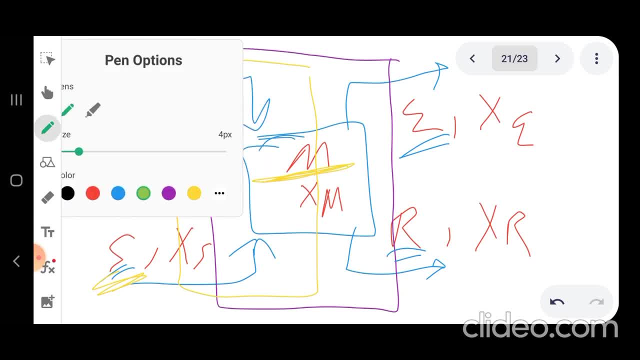 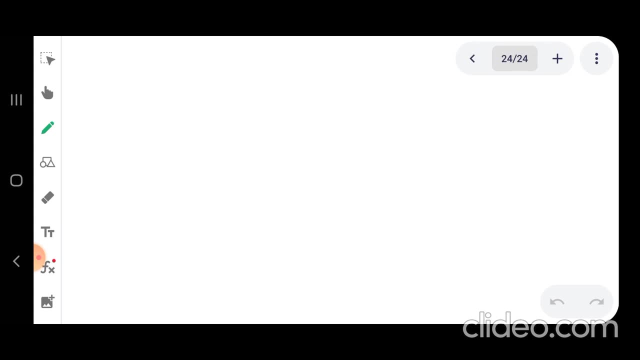 if you would like to focus on this system. so you have what you have: this m equal to e plus r. so usually I like to write it in this way. I like to write it in this way: f plus s equal to m, equal to e plus r. so let's read it together. 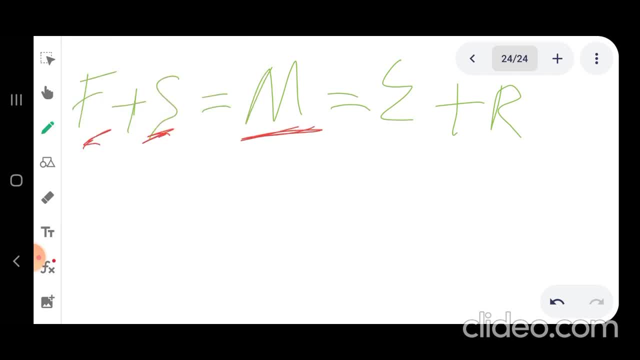 feed plus solvent will be mixed to form a mixture inside the vessel. then you will get two streams: one is the extract and one in the raffinate. this is the overall material balance and similarly you can write component material balance. so x f, f plus x s, s gives you x m, m, gives you x e, e plus x r r. 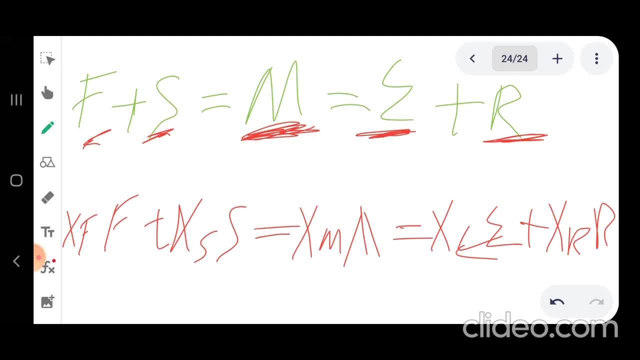 yeah, that's it. so this is the material balance, and we are going to need this material balance later. okay, I'm going to need it later, okay. another thing that I would like to mention here before, before we end up with this video, is that, remember, in distillation, 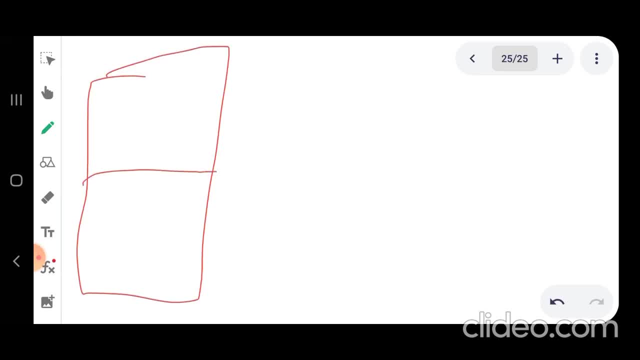 you have two bases, right, you have vapor phase and you have liquid base and within this phase you have A and B. within liquid phase, again, you have A and B and the composition of the vapor phase- remember we called it Y- and composition in the liquid phase, we called it X. and this X and Y, they are referred to by default to 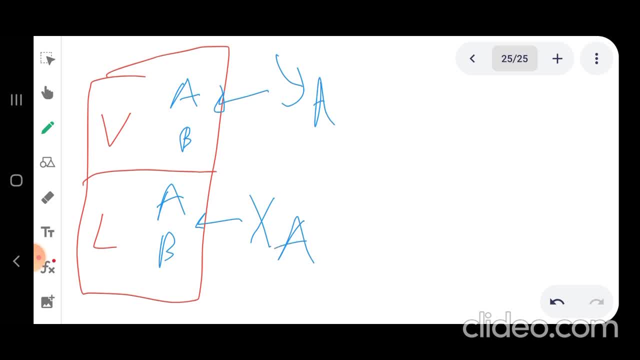 A, which is the more volatile component. okay, so when we just say Y and X- Y means composition of A in the vapor phase, X means composition of A in the liquid phase- then we can represent it graphically using this graph. if you remember X and Y graph, where you draw 45 degree line and then you draw, you draw. 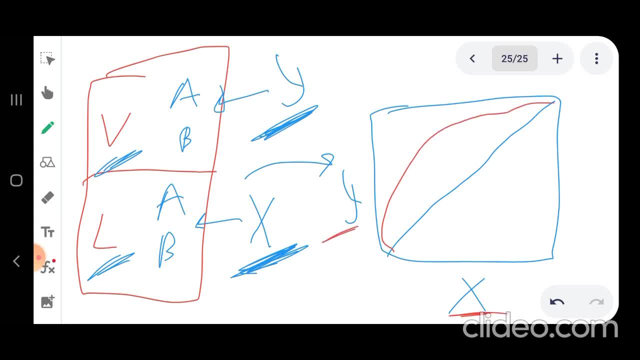 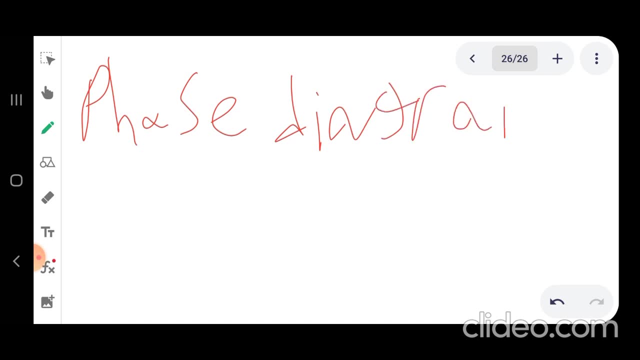 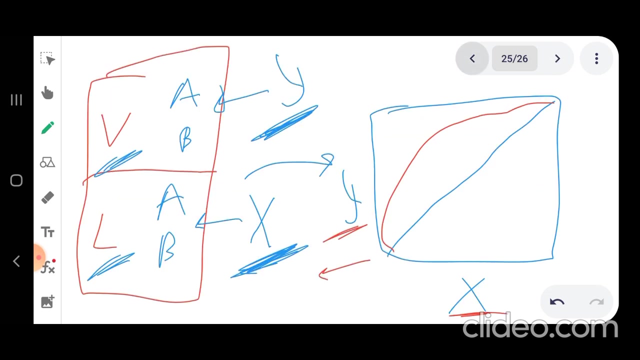 equilibrium curve between X and Y. this diagram, we call it, we call it VAPORFACE, VAPORFACE diagram, we call it VAPORFACE diagram, we call it VAPORFACE diagram. okay, yeah, this diagram, we call it a VAPORFACE diagram, which is nothing but a simple diagram. 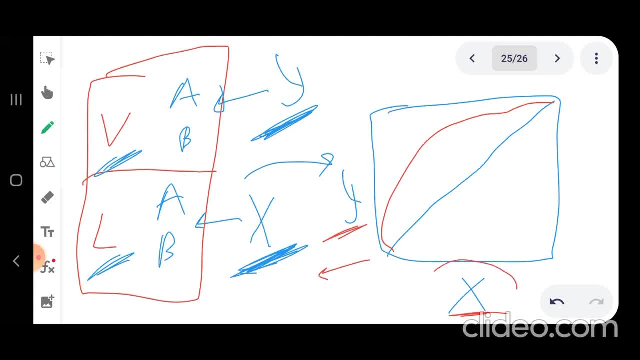 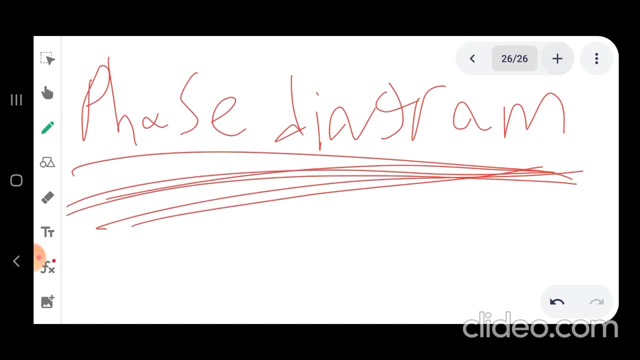 that's drawn between composition in one VAPORFACE and composition of another VAPORFACE, in this case for distillation. they are composition of liquid VAPORFACE and VAPORFACE now, similarly in extraction. can we have a VAPORFACE diagram? yes, we can. we can have a VAPORFACE diagram again. this VAPORFACE diagram is: 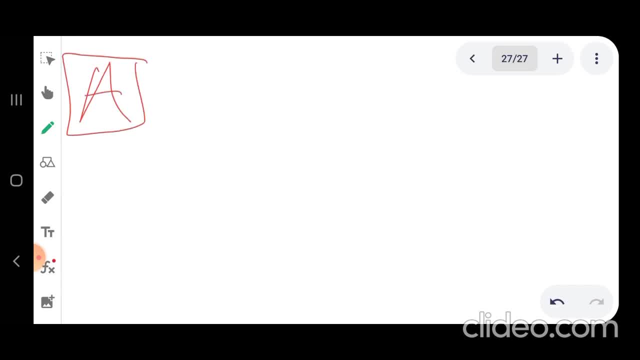 based on component A, which is the solute in this case. in this case, it is the solute for extraction. so again, but the problem here? do we have vapor and liquid? no, here we have a liquid and liquid. okay, so we need to draw this diagram between two vases, but what are? 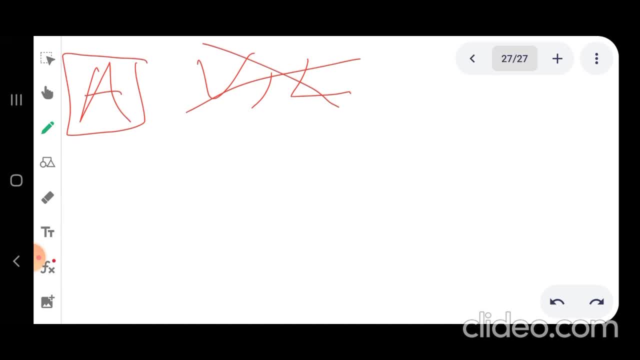 these two vases, simply they are. simply they are extract and raffinate vases. see these two vases, extract and raffinate. so you have what you have, extract these and you have raffinate vase. we don't have here liquid and vapor, no, we have liquid and liquid. 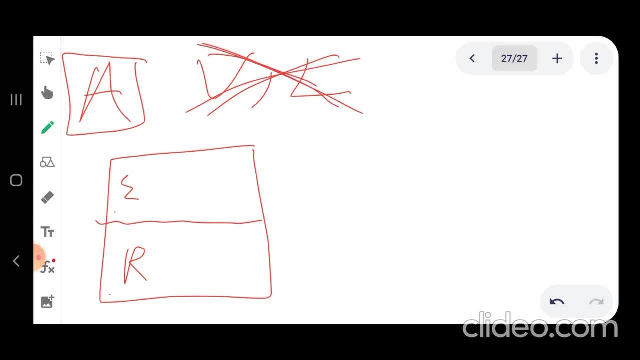 but they are two different liquids. remember the example of oil and water when we say water is heavier, so it would go down, oil is lighter, so it will go up. same thing- up will go down as well- applies here. here we have an extract and raffinate this, raffinate with the composition xr and this. 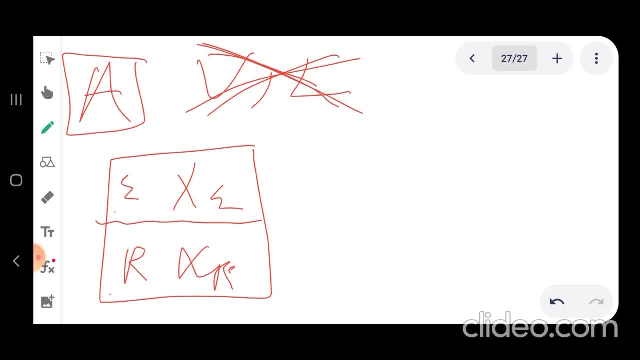 extract with the composition xe. again, these two bases, these two compositions are referred to solute a, solute a. so we can draw same diagram, but instead of x and y we will draw it between xr and xe, raffinate composition and extract composition. and again we can draw our 45 degree line and then we can draw the equilibrium line which is: 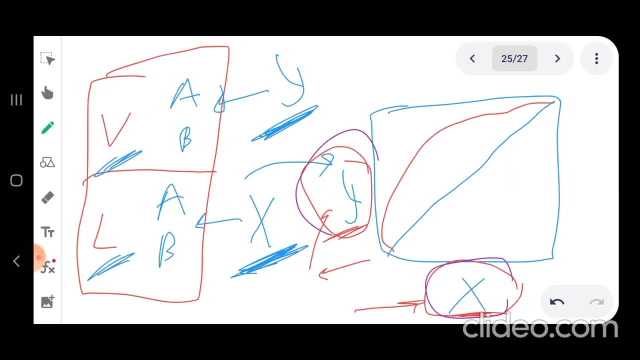 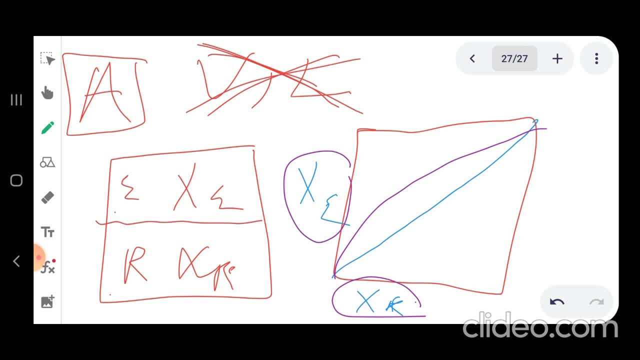 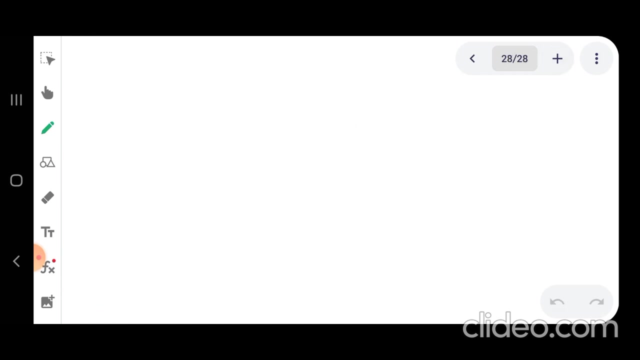 instead of being between x and y, it will be between xr and xe. composition in raffinate base and composition and extract base. okay, so this is again what we call that base diagram: base diagram between two bases: raffinate and extract. okay, so this is one diagram. another famous diagram- it's new to you, i think- is called components. 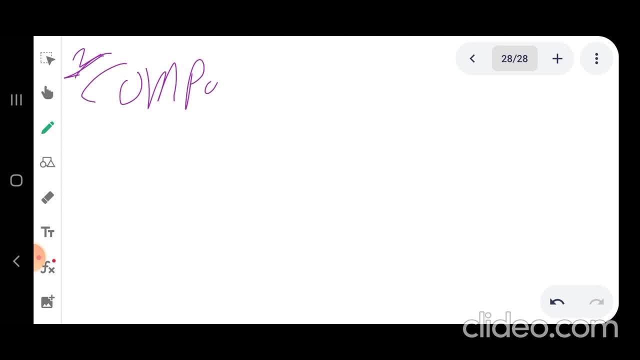 so this is the second one, components diagram. this diagram is drawn between the three components we have remember. remember, we have a ternary system. we have a ternary system where we have three components. we have three components which are: so, again, we have two bases: extract and raffinate. but we have 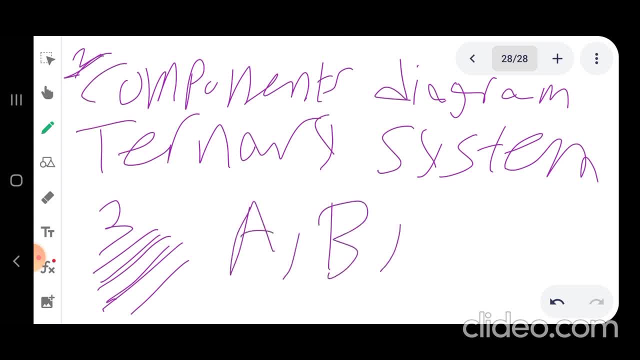 components, which are a, b and c. as we said before, a is solute, b is solvent, c is carrier. okay, so can we draw this component diagram? but wait a minute. i mean by a component diagram. component diagram is simply a diagram that shows the composition of each of these three components. 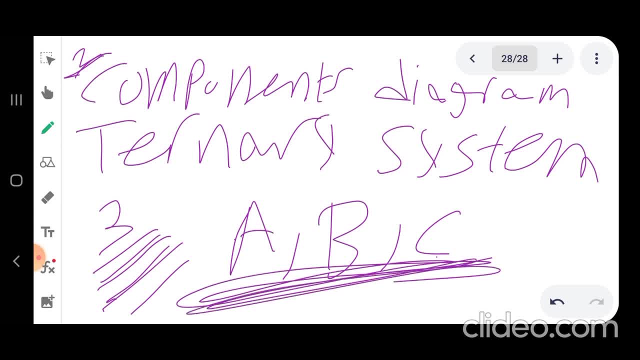 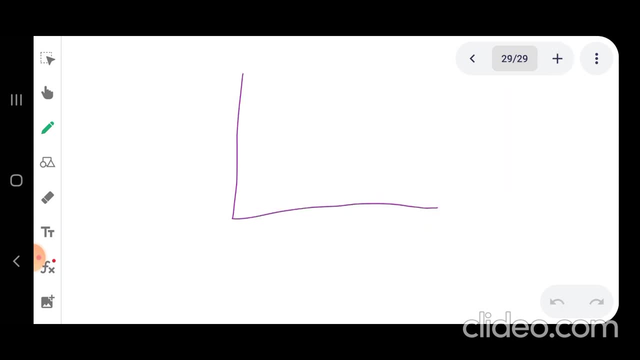 their compositions. okay. so, as you can imagine, we need how many axes, how many components. we have here one, two, three. so we need three axes. we need three axes. let's call them X, Y and Z axis. okay. so let's say, let's say randomly, let's say randomly or yeah. 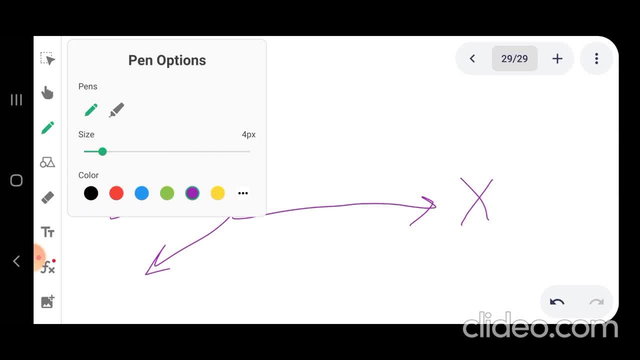 let's say arbitrarily that X is, let's say arbitrarily that X is, is the composition of V's. for example, a represent composition of these, a and Y represent the composition of these, b & z represent the composition of V, C, okay, okay, so it happens here at this point, the origin. 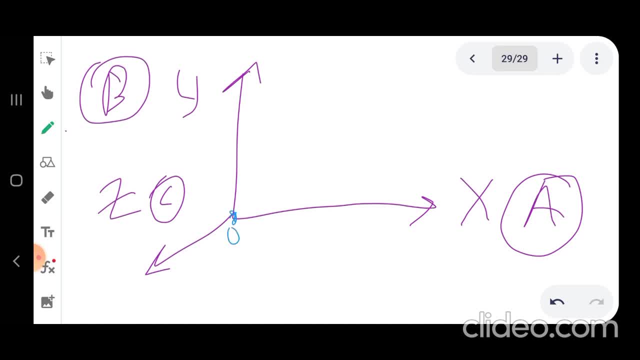 you have zero a zero b 0 C. okay so. you have zero a zero b 0 C, okay so. and then, as you go along the x-axis until the end, you reach a point of 100 percent a. so this is from zero percent to 100 percent a. this is the x-axis. similarly, the y-axis is from: 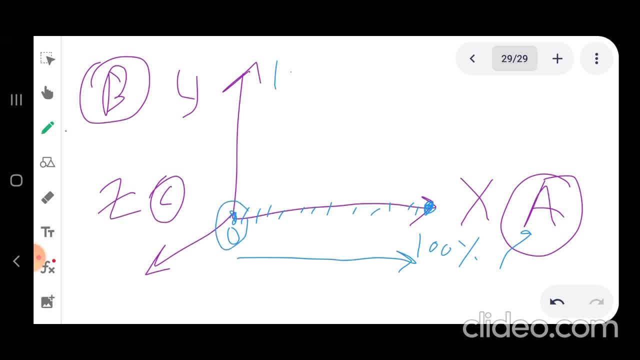 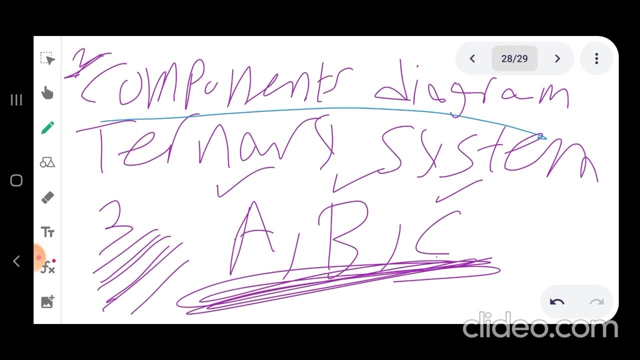 zero percent y up to 100 percent b. so this is along the y-axis, from zero percent b to 100 percent b. similarly, along the z-axis, from zero percent c to 100 percent c. okay, so this is called what this is called: components diagram, but there is a problem here. there is a problem. the problem here is that this diagram 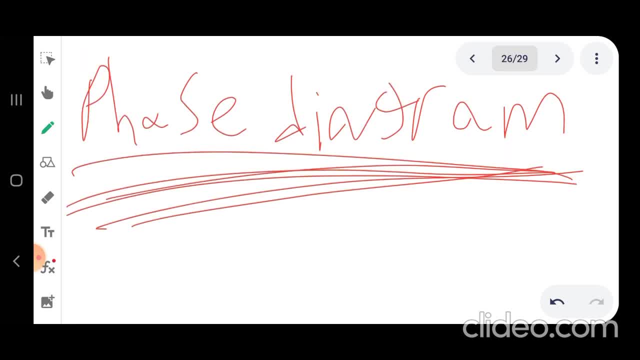 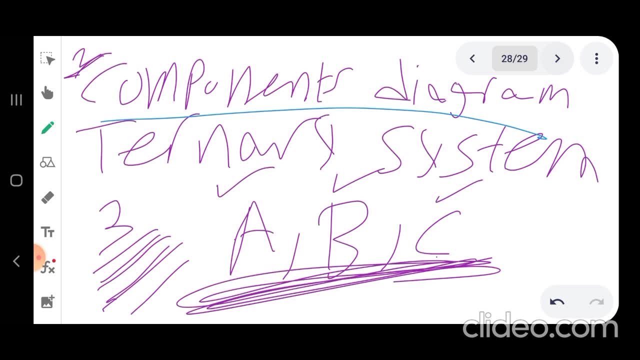 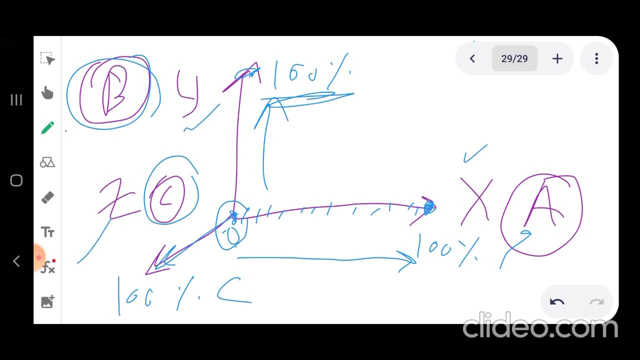 is not like the vase diagram. see the vase diagram. here is two-dimensional, two-dimensional diagram, but here the component diagram is a three-dimensional diagram where you have x, y and z, in other words one axis for a, one axis for b and one axis for z compositions. 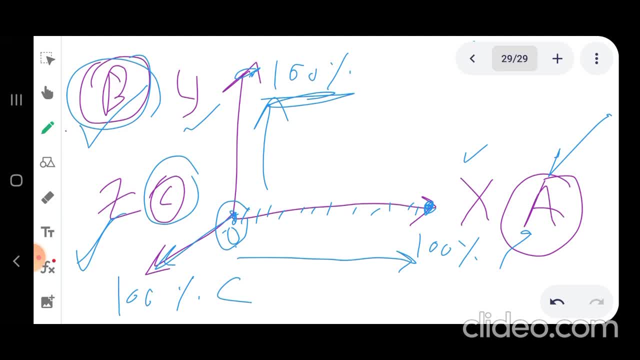 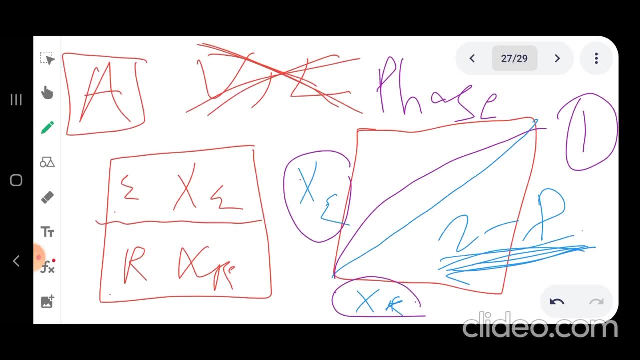 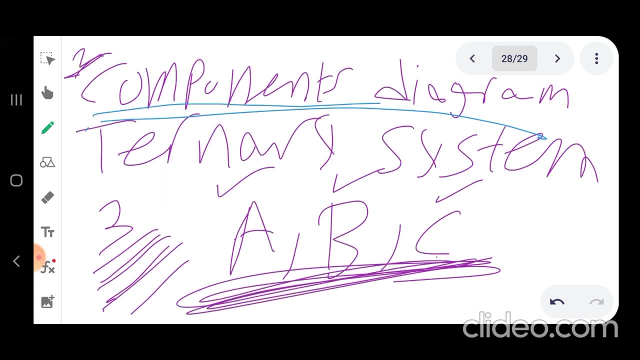 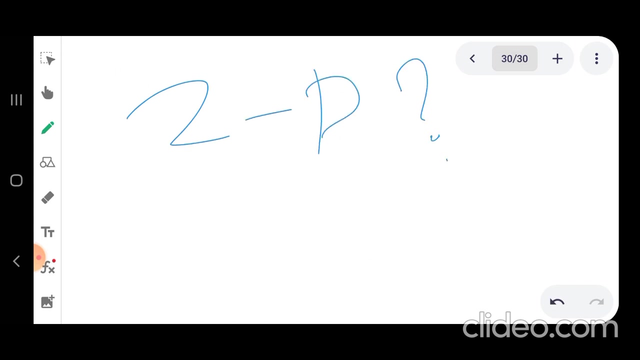 you okay. the problem here is: this is a three-dimensional diagram and the vase diagram is two-dimensional. so the question here: is there a way to represent the components diagram in a two-dimensional form? can we represent this diagram in a two-dimensional form rather than this complicated three-dimensional diagram? 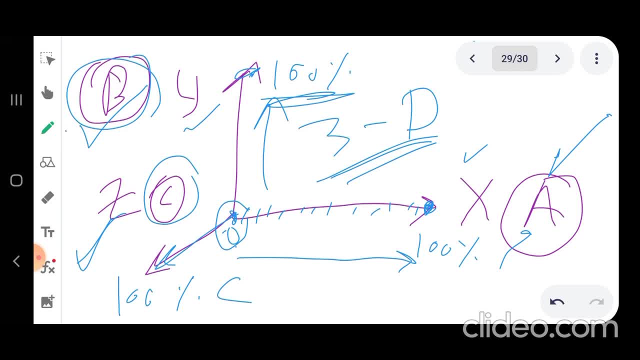 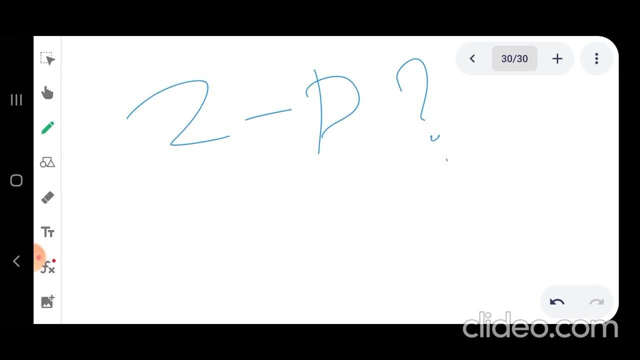 the answer is yes. mathematicians has came up with a brilliant idea, a brilliant idea which is the triangular diagrams. the triangular diagrams, which has mainly two types, this two-dimensional diagram. it could be equilateral diagram, or it could be upright diagram, upright triangular diagram. okay, as you can see, these diagrams are two-dimensional. 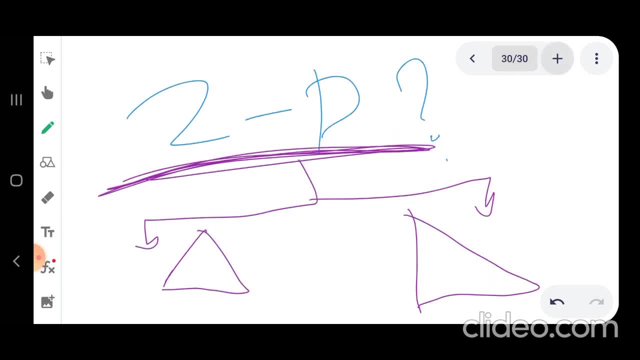 they are not three-dimensional, they are two-dimensional, and so it could be equilateral or triangular, upright triangular diagram. again, it could be equilateral triangular diagram or upright- upright means 90 degree triangular diagram. in this course, i'm going to focus only on this type, which is the upright wet. 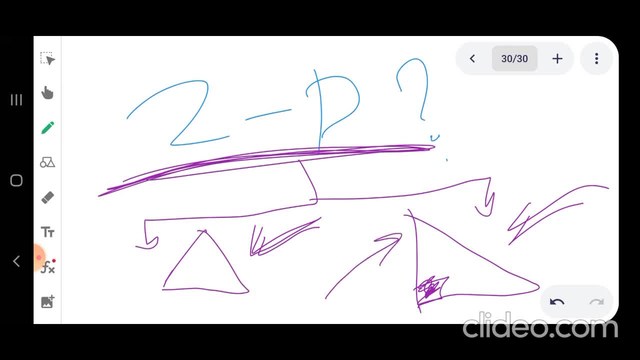 on this course. i m going to focus only on this type, which is the upper of currently. Booth will use the upright, so I envelope. you can use No, which would give you the same answer, but I feel this is simpler to millions. I would say that because, uh, interesting. I would better to enter the points. ah, I think it would make quite a bit of difference. after a presentation, I would choose to be able to answer all these points together instead of highlighting the top and the bottom charts. I think this will be a really useful tool for you. 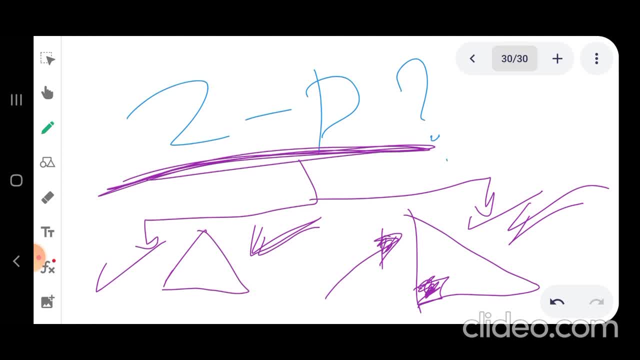 tendency to what questionhoovers can put in the future, if you want to keep up to date or other exercises of this course I discuss. this is simpler to understand- an upright triangular diagram, so I'm going to focus on this type of diagrams. okay, so what this diagram is? simply, it is you. 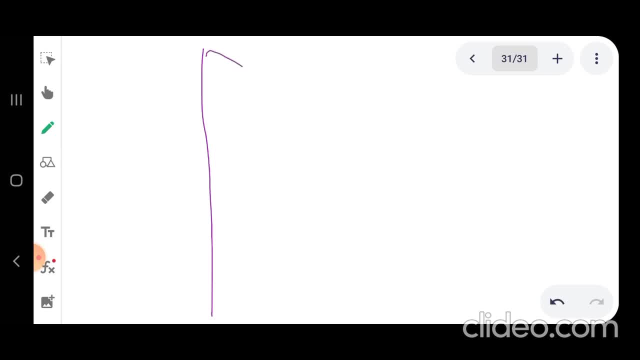 draw this 90 degree. you draw this 90 degree. so I angle. let me do it like this: we draw this 90 degree triangle and again same idea, same idea. this is X axis, this is y axis, this is z axis. but rather than having angle, you need to have diagonal and you need individual heights. 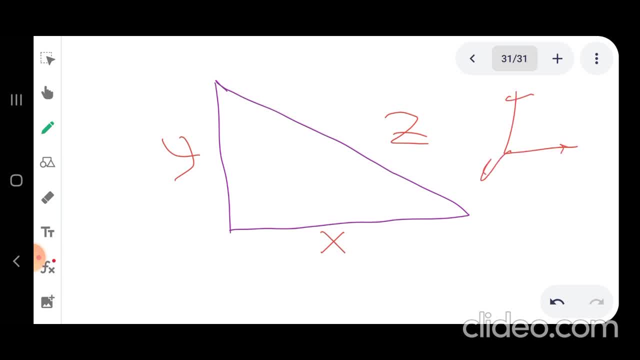 them in a three-dimensional form. no, we draw it in a two-dimensional form to be easier to analyze and solve the problems. okay, so let's see, this is the origin. this is the origin. how many corners we have here in this upright triangle? we have three corners: one. 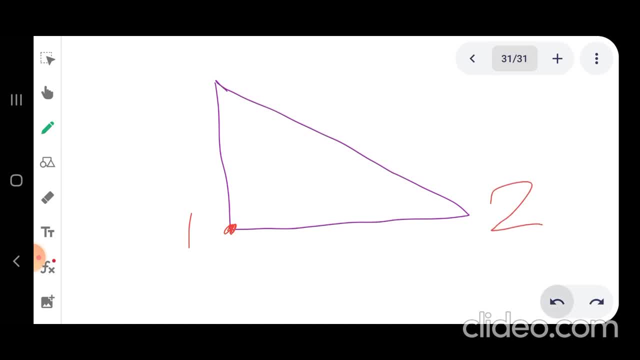 two, three, three corners. okay, so let's call this: corner c refer to component c, and then let's call this: corner b refers to component b, and then let's call this: corner a refers to component a. so let's link to the three-dimensional diagram in the three-dimensional diagram. 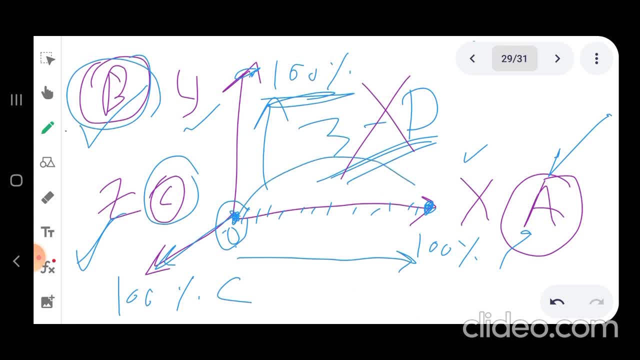 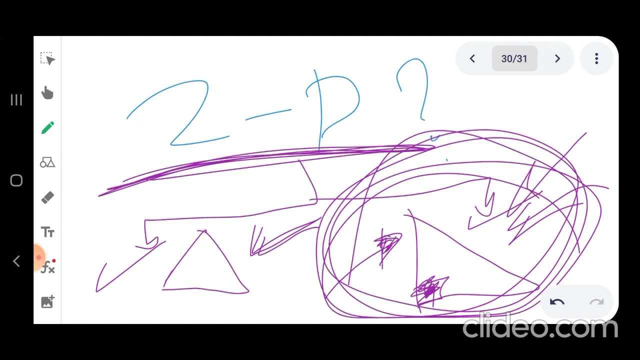 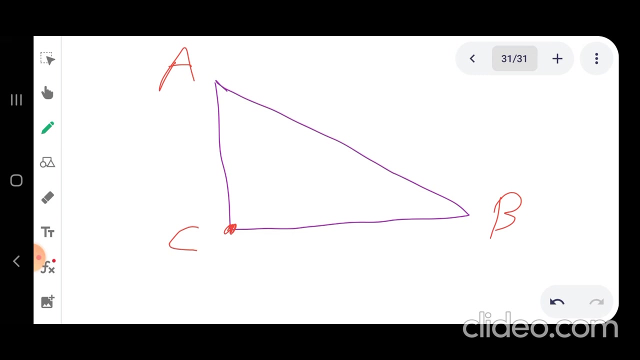 we say from here to here is from 0 to 100% composition, and similar from here to here and here to here, or from 0 to 100% composition of a given component, a, B or C. similarly, here at one of the corners. any corners represent 100%. I in this. 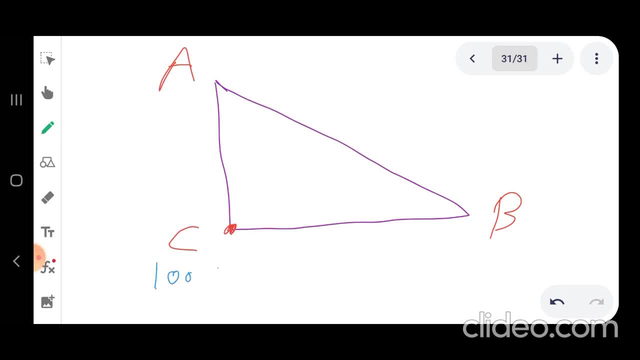 corner it is 100% C. in this corner it is 100% B. in this corner it is 100% A. so you can have this天 reconf HTML video. have this scale: if this is 100% B, so this is 0% B. so from here. 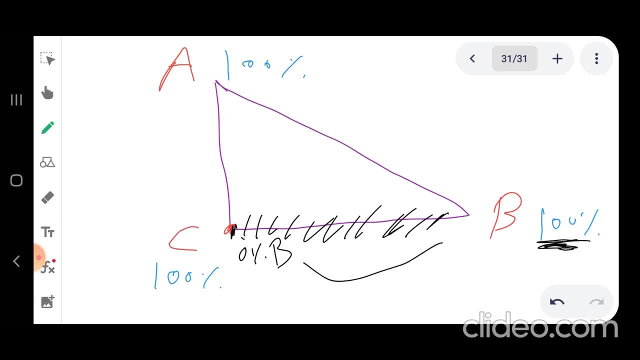 to here or to there. from here to here, it is from zero percent to 100 percent b. okay, and similarly. similarly, if this is 100 percent c, so from here to here, this is zero percent c and this is 100 percent c. from here to here: from here zero percent c and here 100 percent c. and similarly you can extend. 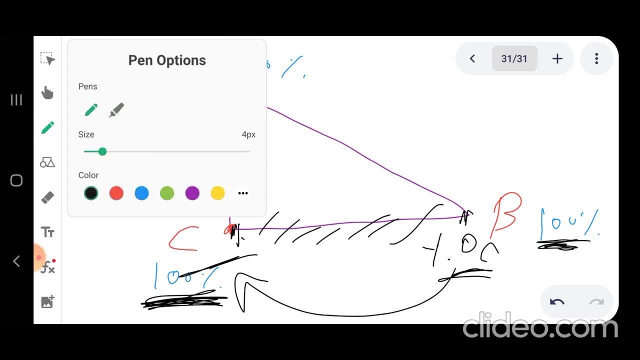 the idea. so, similarly, from here zero percent a and here 100 percent a, and in between you can have, i don't know, 10, 10 percent a, 50 percent a, up to all the way to 100 percent a. okay, and then and vice versa, and vice versa. i. 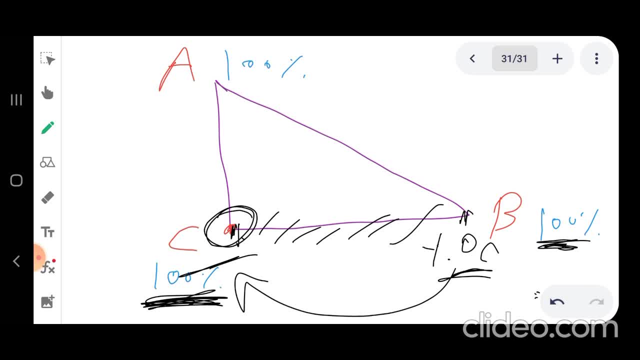 from here is zero percent c and here 100 percent c, so this would be one 10 percent c. i don't know any 50 percent c all the way until you reach this corner where you have 100 percent c, and same idea applies here. from here to here: zero to 100 percent b. from here to there: zero from 100 percent a. okay, so this is. 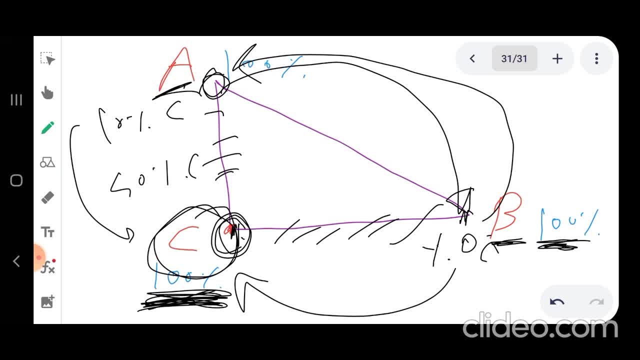 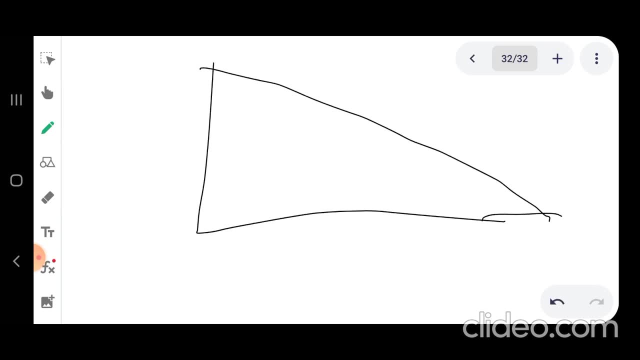 how to how to understand this upright triangular component diagram. okay, so this is your axis. again, you would have this three axis. one of the corner represent 100 percent c, 100% B. this is 100% A. to be consistent, we will always call this. 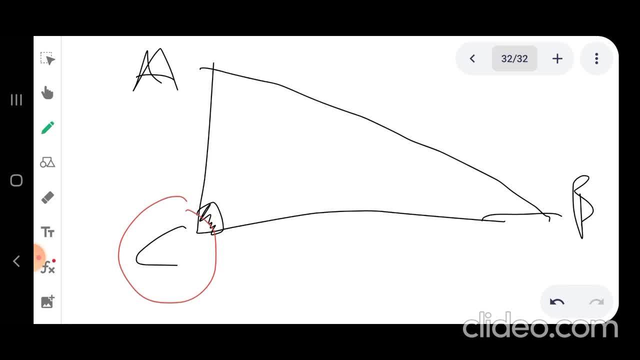 corner C and we will always call this corner B and we will always call this corner A. okay, so this is our axis. then, to draw the equilibrium curve inside it, you needed some data. you need the data. okay, you need a data of composition of A, composition of B and composition of C. you need to have this set of data. it is 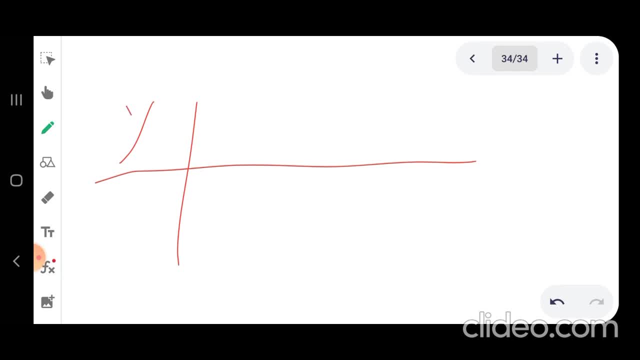 like when you have in distillation. you have X and Y data and then you draw them in XY diagram. similarly, here you need to have composition data of A, B and C and then you can draw them on this triangular diagram. okay, so it is easier. if you want to draw a point, I suppose you. 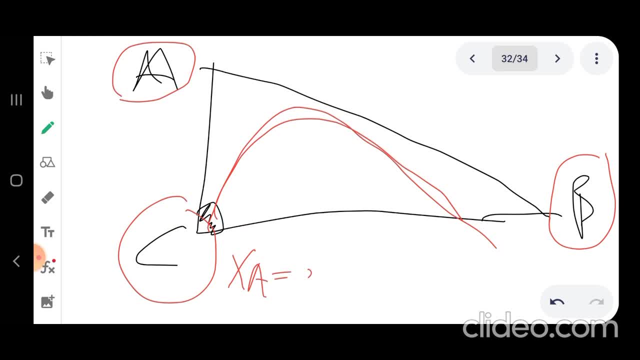 have a point: x a equal to 0.1 and x b is equal to 0.2 and x c is equal to 0.7. so it is easier. it is easier to look at. don't look at this axis, look only at these two axes to make. 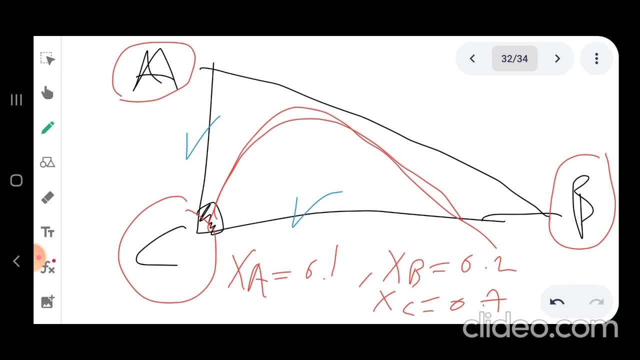 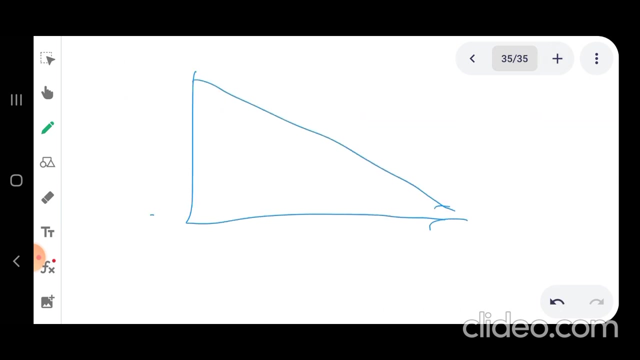 things simple. this axis represents 0 b up to 100 b and this axis represent 0 a up to 100 a. okay, so what you will do, let me do it again. this is c, this is b, this is a. so suppose you have a composition that will say: 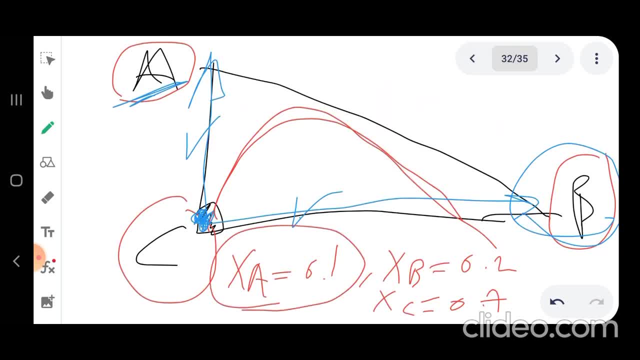 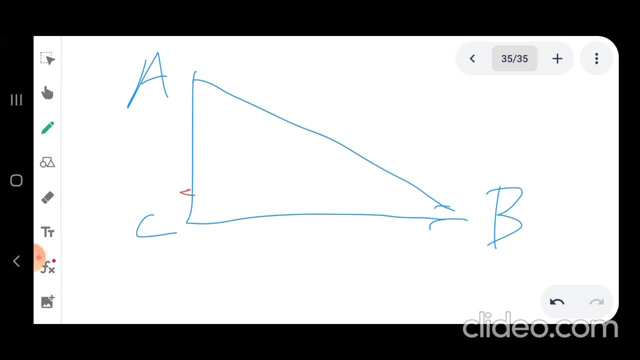 0.1 a, which is 10, and 0.2 b, which is 20, so you don't have to look at c, don't look at this axis, okay, so what you will do, you will look where is 10 a. it is somewhere here, because here is 10 percent is 100 percent a. 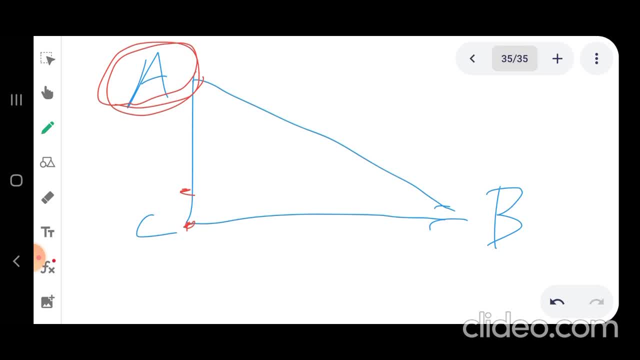 here 0 percent a. in between is, let's say, closer to 0. this is 10 percent a, this is 10 percent a. and then where is your b? here, this is 0 b, here 100 b. so 20 percent b would be some somewhere. 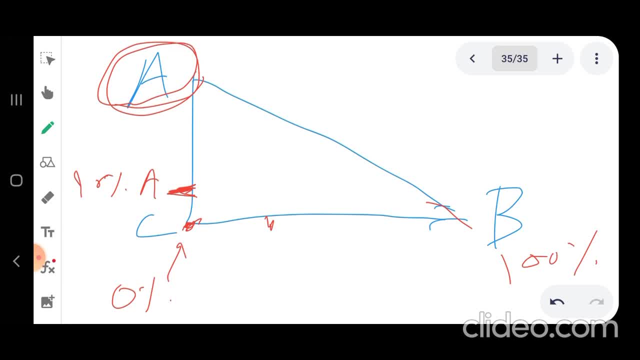 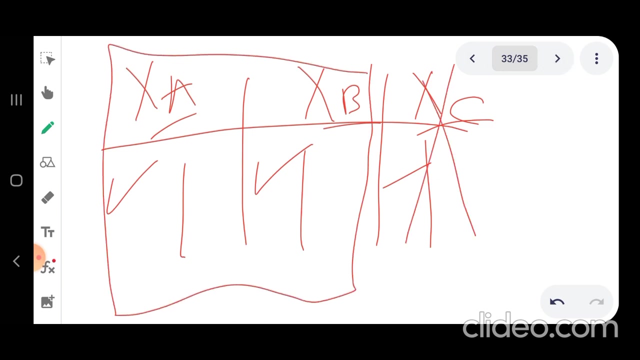 here somewhere. here is 20% B, this is 20% B. okay, so this is your point. this is your point. okay, so you don't have, you don't have to look at C composition. you can draw your curve, equilibrium curve, only by looking at X A and X B. okay, so you can think of this diagram as simple. 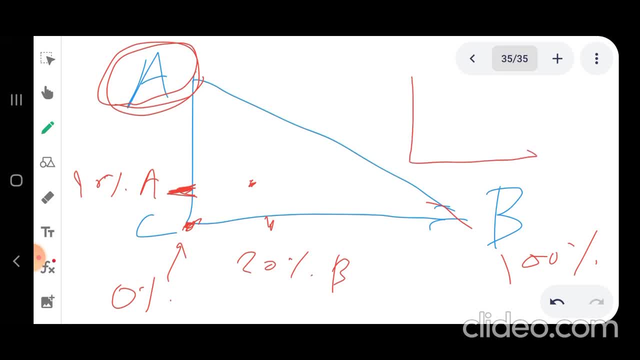 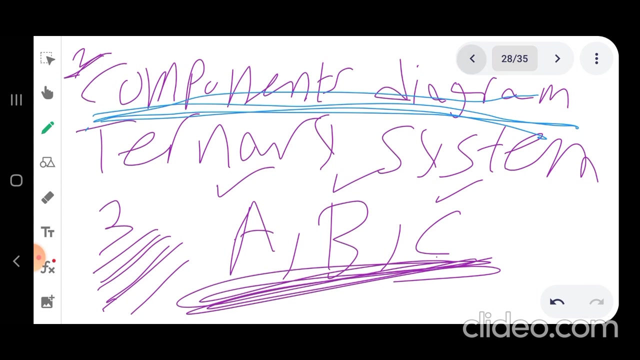 as this as a diagram, as a two-dimensional diagram, where you have here composition from 0 to 100% B and here from 0 to 100% A, and then you can draw your points and then connect them to have the equilibrium curve. and similarly, on the Vase diagram, to draw this vase diagram.